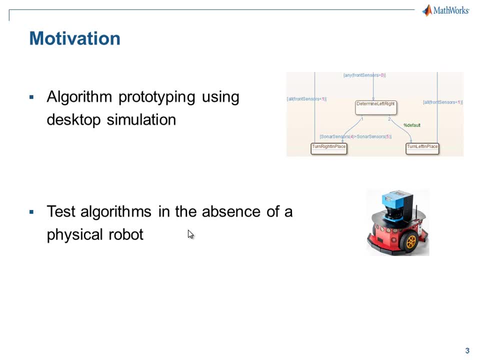 You can also prove this simulation proven algorithm in a real robot as shown in video 2 here, where the real robot is doing obstacle avoidance. You can also prove this simulation proven algorithm in a real robot as shown in video 2 here, where the real robot is doing obstacle avoidance. 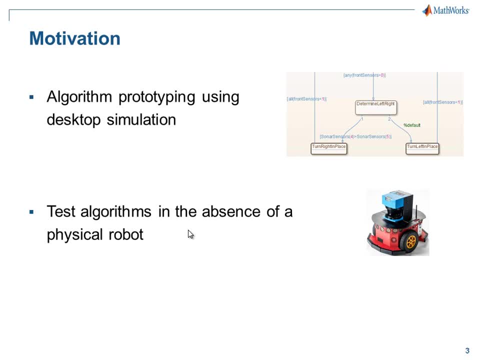 You can also prove this simulation proven algorithm in a real robot as shown in video 2 here, where the real robot is doing obstacle avoidance. You can also prove this simulation proven algorithm in a real robot as shown in video 2 here, where the real robot is doing obstacle avoidance. 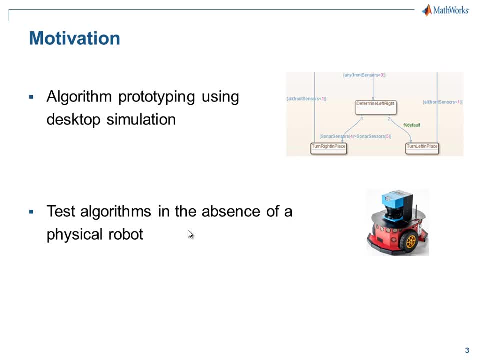 You can also prove this simulation proven algorithm in a real robot as shown in video 2 here, where the real robot is doing obstacle avoidance. You can also prove this simulation proven algorithm in a real robot as shown in video 2 here, where the real robot is doing obstacle avoidance. 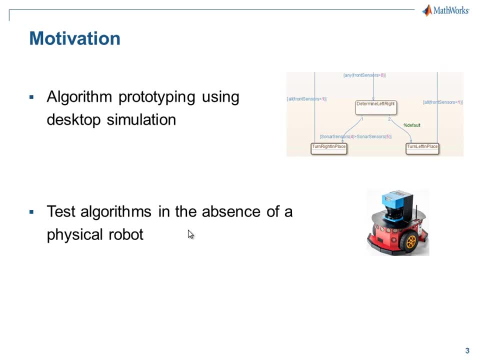 You can also prove this simulation proven algorithm in a real robot as shown in video 2 here, where the real robot is doing obstacle avoidance. You can also prove this simulation proven algorithm in a real robot as shown in video 2 here, where the real robot is doing obstacle avoidance. 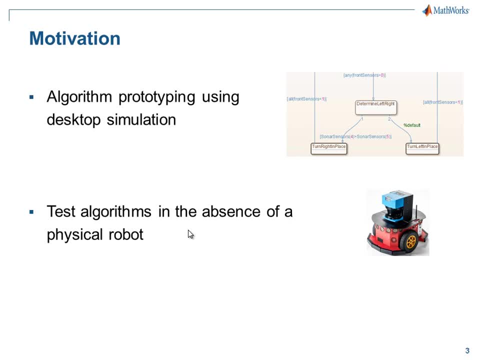 You can also prove this simulation proven algorithm in a real robot as shown in video 2 here, where the real robot is doing obstacle avoidance. You can also prove this simulation proven algorithm in a real robot as shown in video 2 here, where the real robot is doing obstacle avoidance. 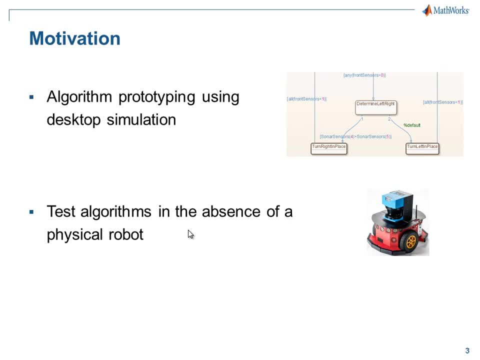 You can also prove this simulation proven algorithm in a real robot as shown in video 2 here, where the real robot is doing obstacle avoidance. You can also prove this simulation proven algorithm in a real robot as shown in video 2 here, where the real robot is doing obstacle avoidance. 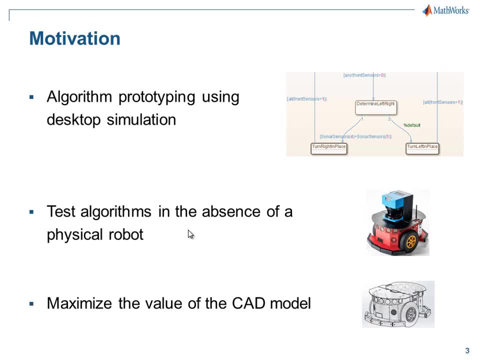 You can also prove this simulation proven algorithm in a real robot as shown in video 2 here, where the real robot is doing obstacle avoidance. You can also prove this simulation proven algorithm in a real robot as shown in video 2 here, where the real robot is doing obstacle avoidance. 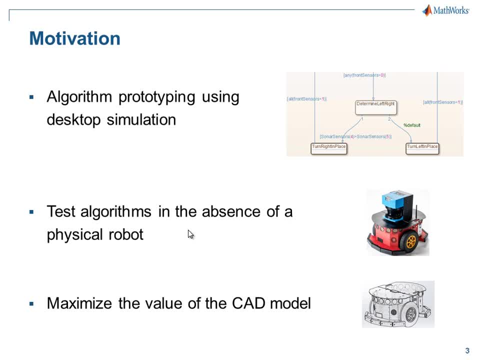 You can also prove this simulation proven algorithm in a real robot as shown in video 2 here, where the real robot is doing obstacle avoidance. You can also prove this simulation proven algorithm in a real robot as shown in video 2 here, where the real robot is doing obstacle avoidance. 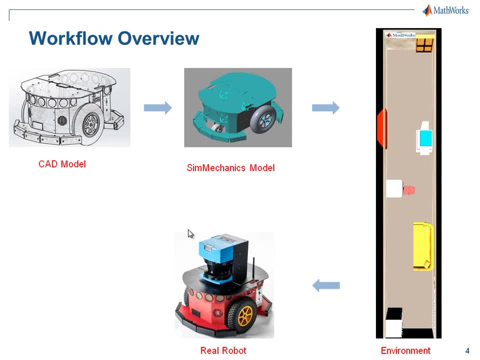 You can also prove this simulation proven algorithm in a real robot as shown in video 2 here, where the real robot is doing obstacle avoidance. You can also prove this simulation proven algorithm in a real robot as shown in video 2 here, where the real robot is doing obstacle avoidance. 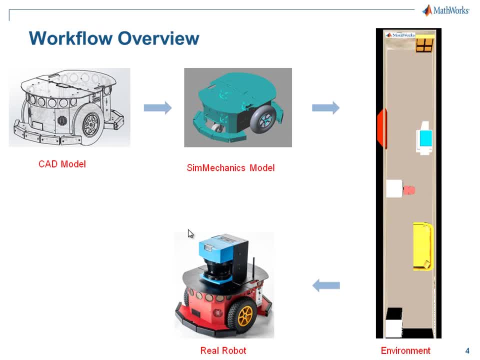 You can also prove this simulation proven algorithm in a real robot as shown in video 2 here, where the real robot is doing obstacle avoidance. You can also prove this simulation proven algorithm in a real robot as shown in video 2 here, where the real robot is doing obstacle avoidance. 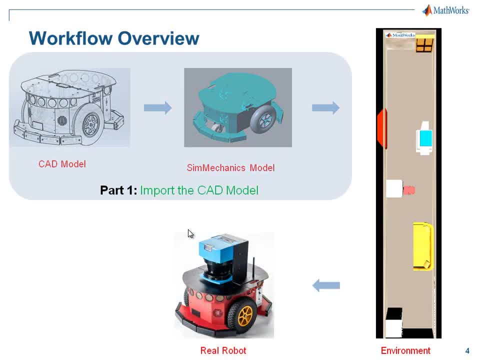 You can also prove this simulation proven algorithm in a real robot as shown in video 2 here, where the real robot is doing obstacle avoidance. You can also prove this simulation proven algorithm in a real robot as shown in video 2 here, where the real robot is doing obstacle avoidance. 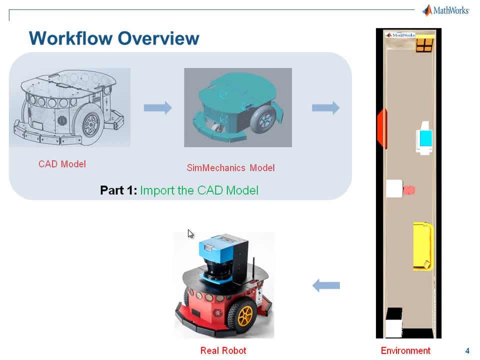 You can also prove this simulation proven algorithm in a real robot as shown in video 2 here, where the real robot is doing obstacle avoidance. You can also prove this simulation proven algorithm in a real robot as shown in video 2 here, where the real robot is doing obstacle avoidance. 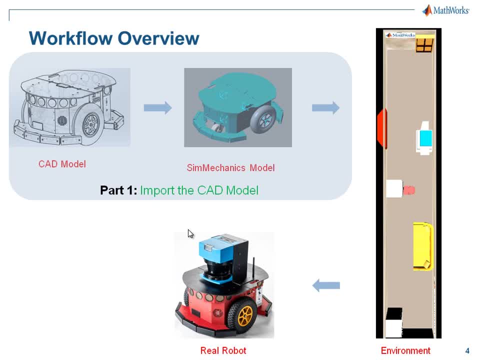 You can also prove this simulation proven algorithm in a real robot as shown in video 2 here, where the real robot is doing obstacle avoidance. You can also prove this simulation proven algorithm in a real robot as shown in video 2 here, where the real robot is doing obstacle avoidance. 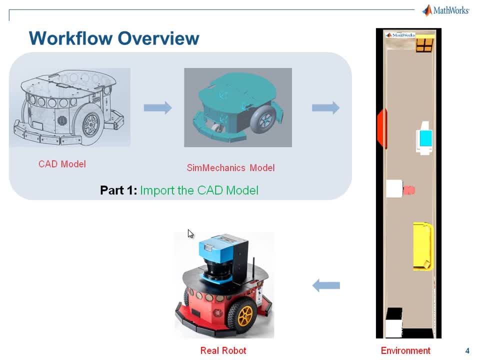 You can also prove this simulation proven algorithm in a real robot as shown in video 2 here, where the real robot is doing obstacle avoidance. You can also prove this simulation proven algorithm in a real robot as shown in video 2 here, where the real robot is doing obstacle avoidance. 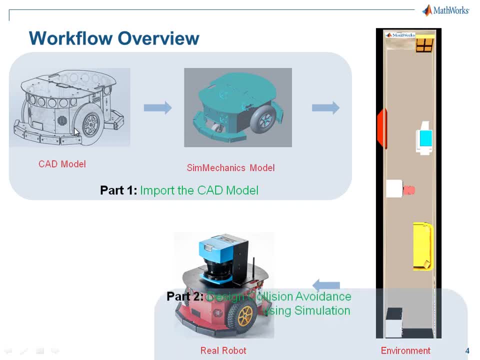 You can also prove this simulation proven algorithm in a real robot as shown in video 2 here, where the real robot is doing obstacle avoidance. You can also prove this simulation proven algorithm in a real robot as shown in video 2 here, where the real robot is doing obstacle avoidance. 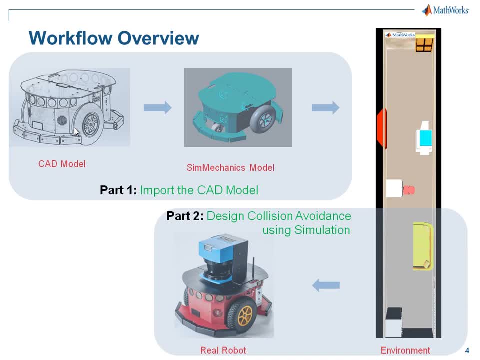 You can also prove this simulation proven algorithm in a real robot as shown in video 2 here, where the real robot is doing obstacle avoidance. You can also prove this simulation proven algorithm in a real robot as shown in video 2 here, where the real robot is doing obstacle avoidance. 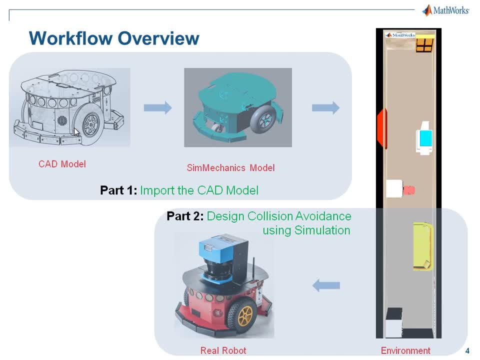 You can also prove this simulation proven algorithm in a real robot as shown in video 2 here, where the real robot is doing obstacle avoidance. You can also prove this simulation proven algorithm in a real robot as shown in video 2 here, where the real robot is doing obstacle avoidance. 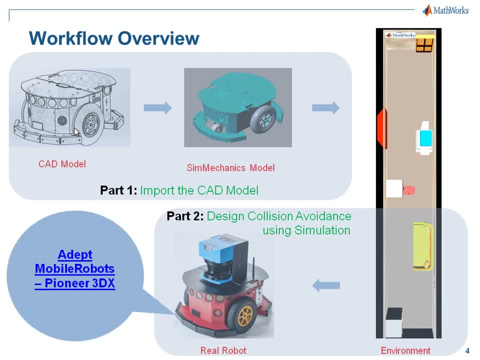 You can also prove this simulation proven algorithm in a real robot as shown in video 2 here, where the real robot is doing obstacle avoidance. You can also prove this simulation proven algorithm in a real robot as shown in video 2 here, where the real robot is doing obstacle avoidance. 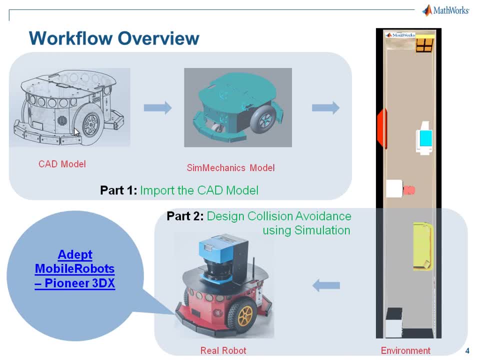 You can also prove this simulation proven algorithm in a real robot as shown in video 2 here, where the real robot is doing obstacle avoidance. You can also prove this simulation proven algorithm in a real robot as shown in video 2 here, where the real robot is doing obstacle avoidance. 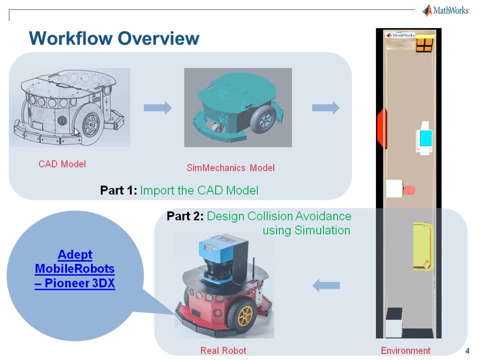 You can also prove this simulation proven algorithm in a real robot as shown in video 2 here, where the real robot is doing obstacle avoidance. You can also prove this simulation proven algorithm in a real robot as shown in video 2 here, where the real robot is doing obstacle avoidance. 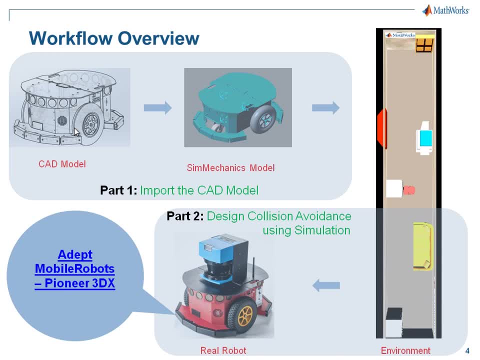 You can also prove this simulation proven algorithm in a real robot as shown in video 2 here, where the real robot is doing obstacle avoidance. You can also prove this simulation proven algorithm in a real robot as shown in video 2 here, where the real robot is doing obstacle avoidance. 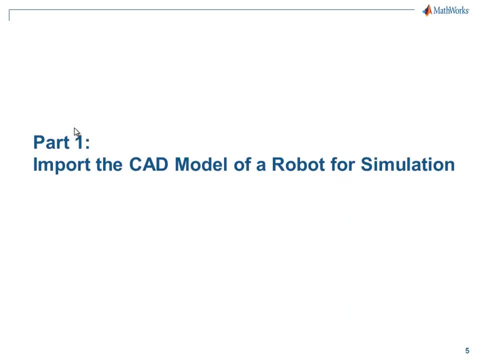 You can also prove this simulation proven algorithm in a real robot as shown in video 2 here, where the real robot is doing obstacle avoidance. You can also prove this simulation proven algorithm in a real robot as shown in video 2 here, where the real robot is doing obstacle avoidance. 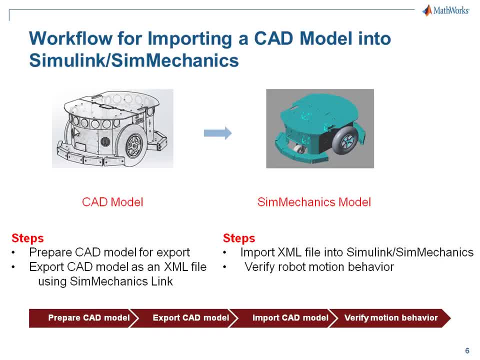 You can also prove this simulation proven algorithm in a real robot as shown in video 2 here, where the real robot is doing obstacle avoidance. You can also prove this simulation proven algorithm in a real robot as shown in video 2 here, where the real robot is doing obstacle avoidance. 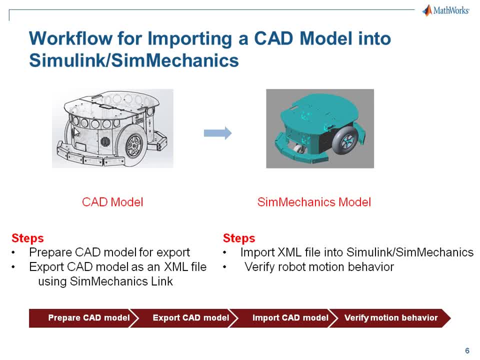 You can also prove this simulation proven algorithm in a real robot as shown in video 2 here, where the real robot is doing obstacle avoidance. You can also prove this simulation proven algorithm in a real robot as shown in video 2 here, where the real robot is doing obstacle avoidance. 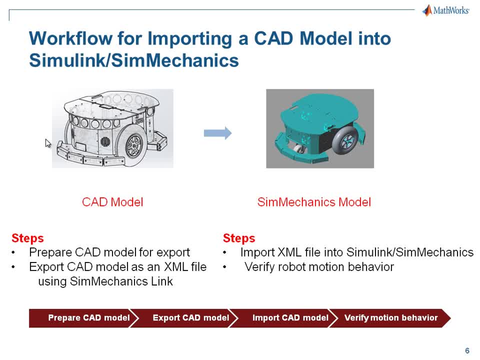 You can also prove this simulation proven algorithm in a real robot as shown in video 2 here, where the real robot is doing obstacle avoidance. You can also prove this simulation proven algorithm in a real robot as shown in video 2 here, where the real robot is doing obstacle avoidance. 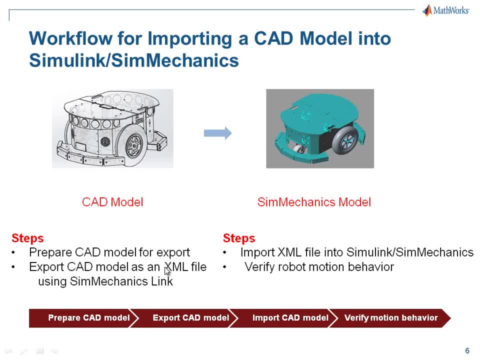 You can also prove this simulation proven algorithm in a real robot as shown in video 2 here, where the real robot is doing obstacle avoidance. You can also prove this simulation proven algorithm in a real robot as shown in video 2 here, where the real robot is doing obstacle avoidance. 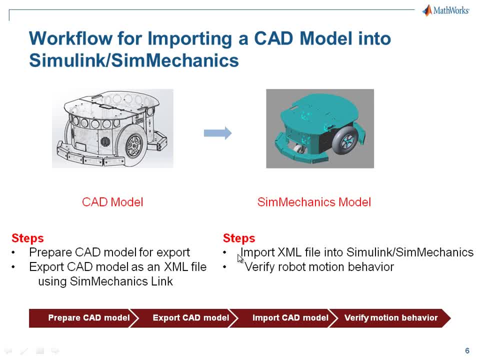 You can also prove this simulation proven algorithm in a real robot as shown in video 2 here, where the real robot is doing obstacle avoidance. You can also prove this simulation proven algorithm in a real robot as shown in video 2 here, where the real robot is doing obstacle avoidance. 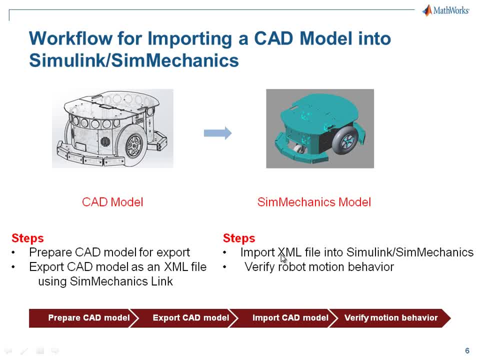 You can also prove this simulation proven algorithm in a real robot as shown in video 2 here, where the real robot is doing obstacle avoidance. You can also prove this simulation proven algorithm in a real robot as shown in video 2 here, where the real robot is doing obstacle avoidance. 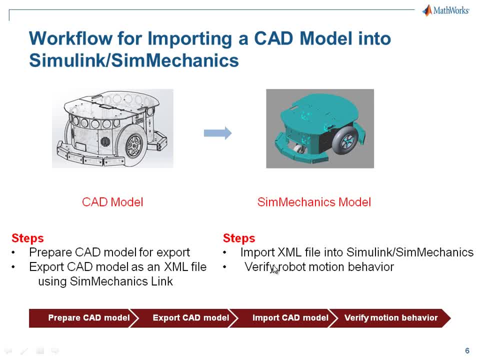 You can also prove this simulation proven algorithm in a real robot as shown in video 2 here, where the real robot is doing obstacle avoidance. You can also prove this simulation proven algorithm in a real robot as shown in video 2 here, where the real robot is doing obstacle avoidance. 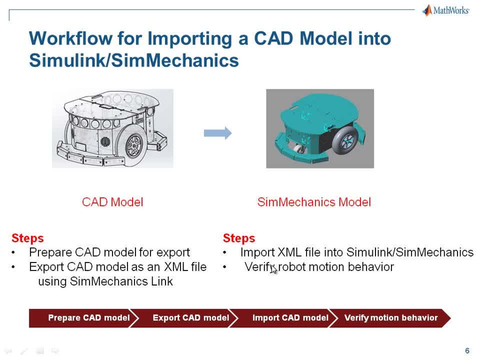 You can also prove this simulation proven algorithm in a real robot as shown in video 2 here, where the real robot is doing obstacle avoidance. You can also prove this simulation proven algorithm in a real robot as shown in video 2 here, where the real robot is doing obstacle avoidance. 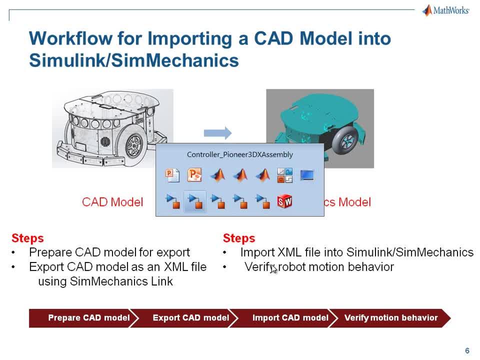 You can also prove this simulation proven algorithm in a real robot as shown in video 2 here, where the real robot is doing obstacle avoidance. You can also prove this simulation proven algorithm in a real robot as shown in video 2 here, where the real robot is doing obstacle avoidance. 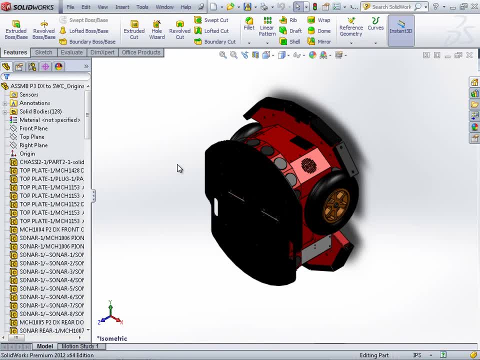 You can also prove this simulation proven algorithm in a real robot as shown in video 2 here, where the real robot is doing obstacle avoidance. You can also prove this simulation proven algorithm in a real robot as shown in video 2 here, where the real robot is doing obstacle avoidance. 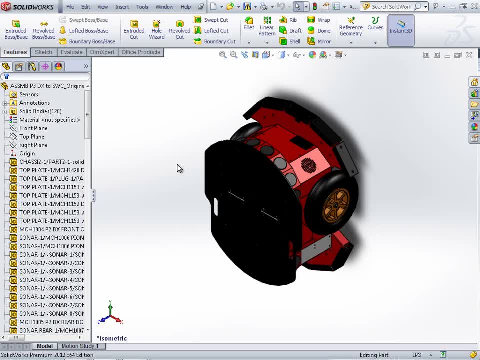 You can also prove this simulation proven algorithm in a real robot as shown in video 2 here, where the real robot is doing obstacle avoidance. You can also prove this simulation proven algorithm in a real robot as shown in video 2 here, where the real robot is doing obstacle avoidance. 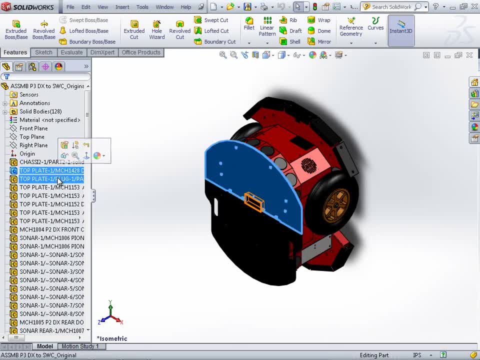 You can also prove this simulation proven algorithm in a real robot as shown in video 2 here, where the real robot is doing obstacle avoidance. You can also prove this simulation proven algorithm in a real robot as shown in video 2 here, where the real robot is doing obstacle avoidance. 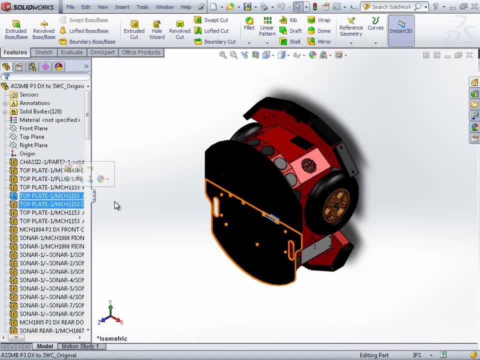 You can also prove this simulation proven algorithm in a real robot as shown in video 2 here, where the real robot is doing obstacle avoidance. You can also prove this simulation proven algorithm in a real robot as shown in video 2 here, where the real robot is doing obstacle avoidance. 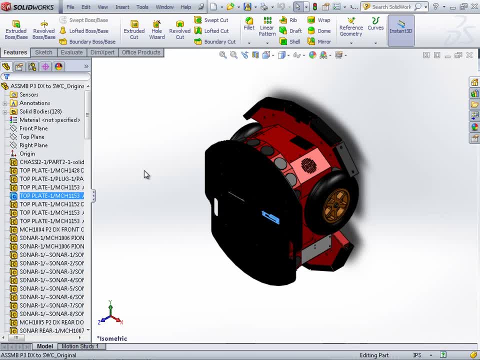 You can also prove this simulation proven algorithm in a real robot as shown in video 2 here, where the real robot is doing obstacle avoidance. You can also prove this simulation proven algorithm in a real robot as shown in video 2 here, where the real robot is doing obstacle avoidance. 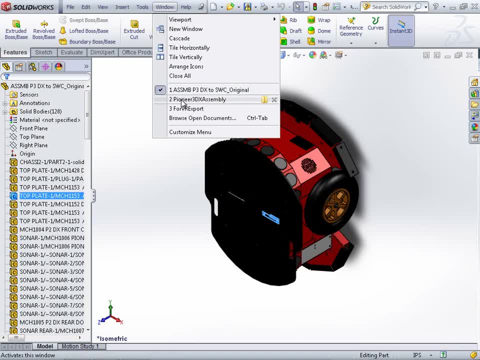 You can also prove this simulation proven algorithm in a real robot as shown in video 2 here, where the real robot is doing obstacle avoidance. You can also prove this simulation proven algorithm in a real robot as shown in video 2 here, where the real robot is doing obstacle avoidance. 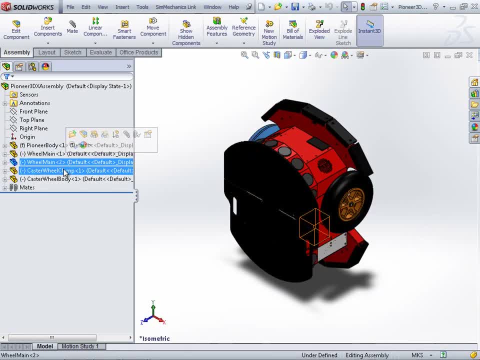 You can also prove this simulation proven algorithm in a real robot as shown in video 2 here, where the real robot is doing obstacle avoidance. You can also prove this simulation proven algorithm in a real robot as shown in video 2 here, where the real robot is doing obstacle avoidance. 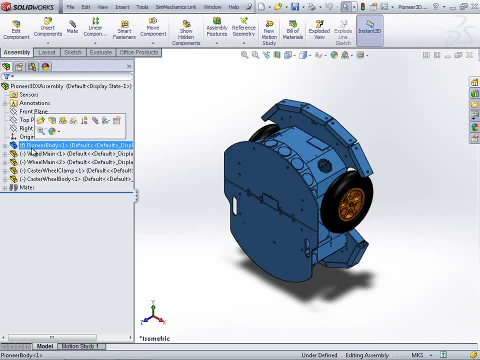 You can also prove this simulation proven algorithm in a real robot as shown in video 2 here, where the real robot is doing obstacle avoidance. You can also prove this simulation proven algorithm in a real robot as shown in video 2 here, where the real robot is doing obstacle avoidance. 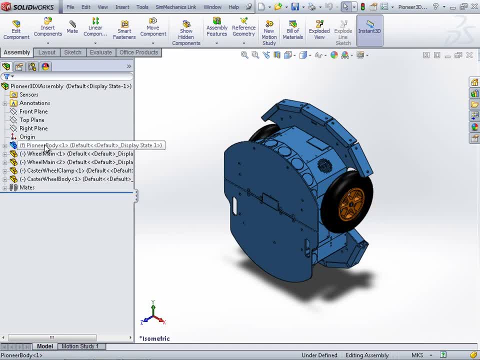 You can also prove this simulation proven algorithm in a real robot as shown in video 2 here, where the real robot is doing obstacle avoidance. You can also prove this simulation proven algorithm in a real robot as shown in video 2 here, where the real robot is doing obstacle avoidance. 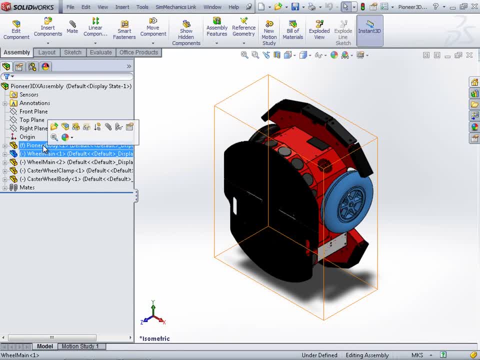 You can also prove this simulation proven algorithm in a real robot as shown in video 2 here, where the real robot is doing obstacle avoidance. You can also prove this simulation proven algorithm in a real robot as shown in video 2 here, where the real robot is doing obstacle avoidance. 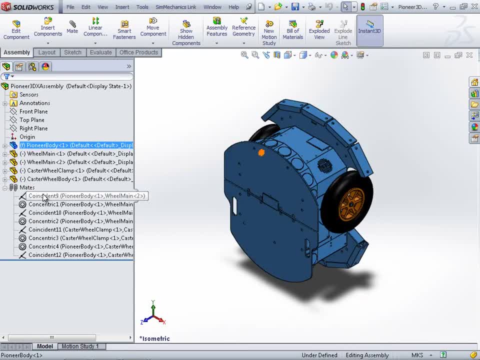 You can also prove this simulation proven algorithm in a real robot as shown in video 2 here, where the real robot is doing obstacle avoidance. You can also prove this simulation proven algorithm in a real robot as shown in video 2 here, where the real robot is doing obstacle avoidance. 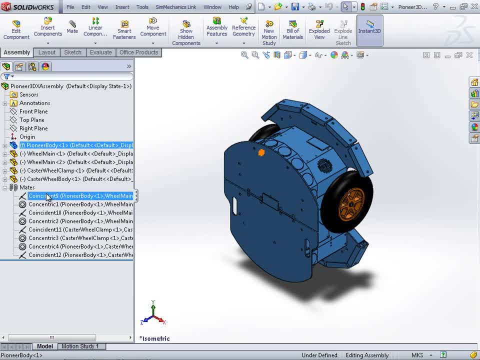 You can also prove this simulation proven algorithm in a real robot as shown in video 2 here, where the real robot is doing obstacle avoidance. You can also prove this simulation proven algorithm in a real robot as shown in video 2 here, where the real robot is doing obstacle avoidance. 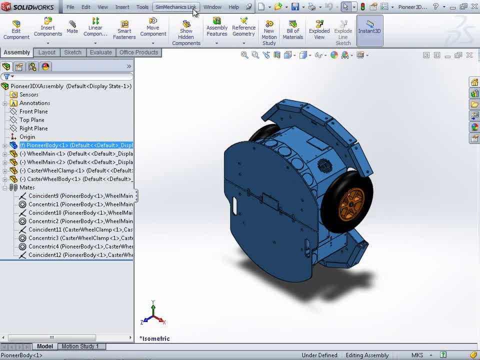 You can also prove this simulation proven algorithm in a real robot as shown in video 2 here, where the real robot is doing obstacle avoidance. You can also prove this simulation proven algorithm in a real robot as shown in video 2 here, where the real robot is doing obstacle avoidance. 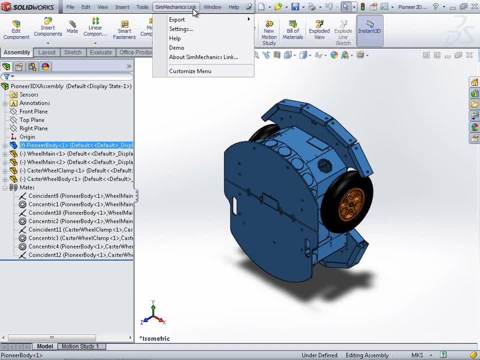 You can also prove this simulation proven algorithm in a real robot as shown in video 2 here, where the real robot is doing obstacle avoidance. You can also prove this simulation proven algorithm in a real robot as shown in video 2 here, where the real robot is doing obstacle avoidance. 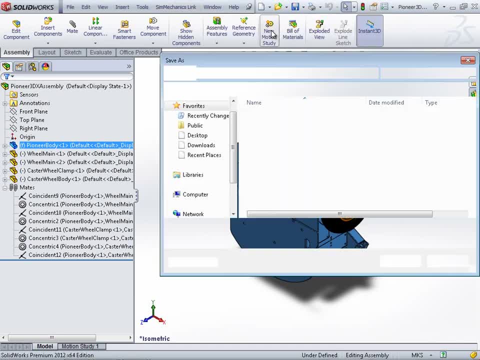 You can also prove this simulation proven algorithm in a real robot as shown in video 2 here, where the real robot is doing obstacle avoidance. You can also prove this simulation proven algorithm in a real robot as shown in video 2 here, where the real robot is doing obstacle avoidance. 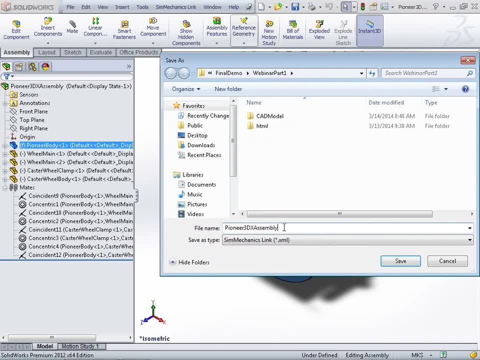 You can also prove this simulation proven algorithm in a real robot as shown in video 2 here, where the real robot is doing obstacle avoidance. You can also prove this simulation proven algorithm in a real robot as shown in video 2 here, where the real robot is doing obstacle avoidance. 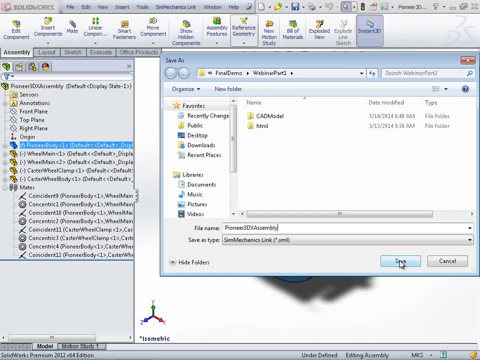 You can also prove this simulation proven algorithm in a real robot as shown in video 2 here, where the real robot is doing obstacle avoidance. You can also prove this simulation proven algorithm in a real robot as shown in video 2 here, where the real robot is doing obstacle avoidance. 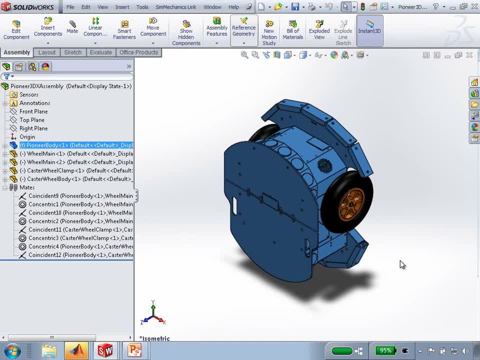 You can also prove this simulation proven algorithm in a real robot as shown in video 2 here, where the real robot is doing obstacle avoidance. You can also prove this simulation proven algorithm in a real robot as shown in video 2 here, where the real robot is doing obstacle avoidance. 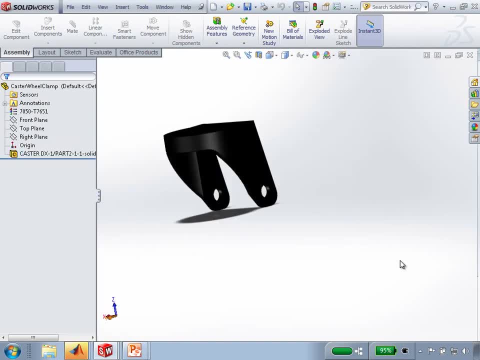 You can also prove this simulation proven algorithm in a real robot as shown in video 2 here, where the real robot is doing obstacle avoidance. You can also prove this simulation proven algorithm in a real robot as shown in video 2 here, where the real robot is doing obstacle avoidance. 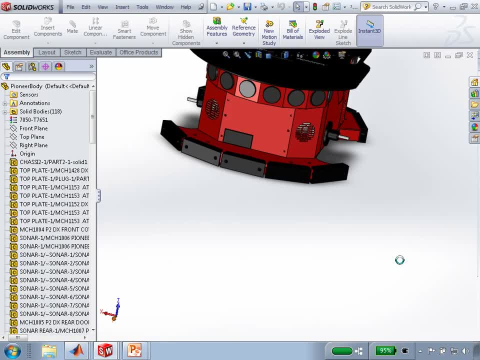 You can also prove this simulation proven algorithm in a real robot as shown in video 2 here, where the real robot is doing obstacle avoidance. You can also prove this simulation proven algorithm in a real robot as shown in video 2 here, where the real robot is doing obstacle avoidance. 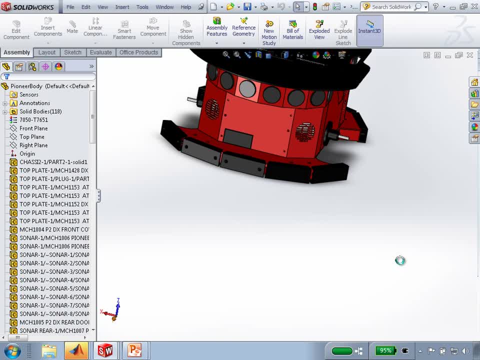 You can also prove this simulation proven algorithm in a real robot as shown in video 2 here, where the real robot is doing obstacle avoidance. You can also prove this simulation proven algorithm in a real robot as shown in video 2 here, where the real robot is doing obstacle avoidance. 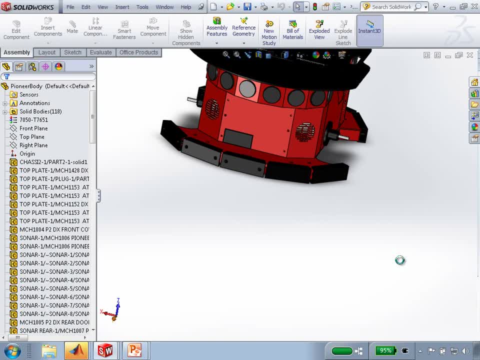 You can also prove this simulation proven algorithm in a real robot as shown in video 2 here, where the real robot is doing obstacle avoidance. You can also prove this simulation proven algorithm in a real robot as shown in video 2 here, where the real robot is doing obstacle avoidance. 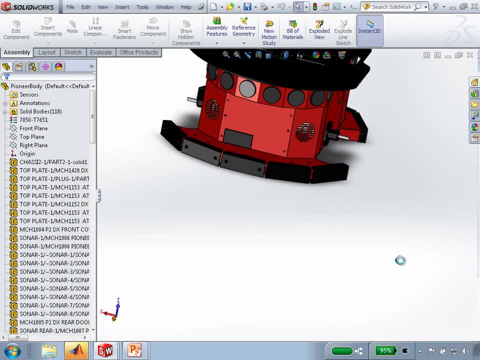 You can also prove this simulation proven algorithm in a real robot as shown in video 2 here, where the real robot is doing obstacle avoidance. You can also prove this simulation proven algorithm in a real robot as shown in video 2 here, where the real robot is doing obstacle avoidance. 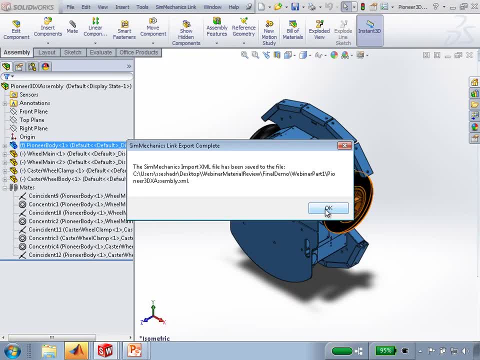 You can also prove this simulation proven algorithm in a real robot as shown in video 2 here, where the real robot is doing obstacle avoidance. You can also prove this simulation proven algorithm in a real robot as shown in video 2 here, where the real robot is doing obstacle avoidance. 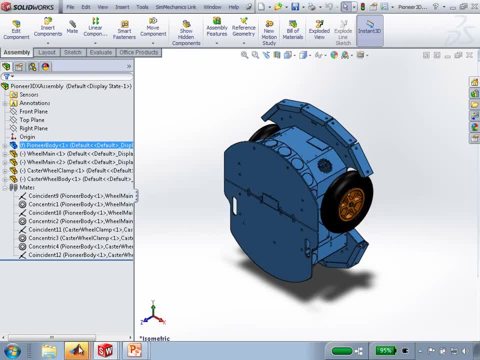 You can also prove this simulation proven algorithm in a real robot as shown in video 2 here, where the real robot is doing obstacle avoidance. You can also prove this simulation proven algorithm in a real robot as shown in video 2 here, where the real robot is doing obstacle avoidance. 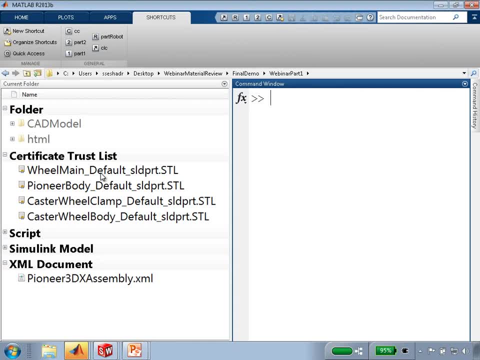 You can also prove this simulation proven algorithm in a real robot as shown in video 2 here, where the real robot is doing obstacle avoidance. You can also prove this simulation proven algorithm in a real robot as shown in video 2 here, where the real robot is doing obstacle avoidance. 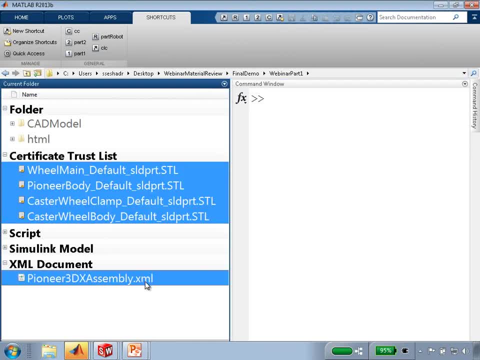 You can also prove this simulation proven algorithm in a real robot as shown in video 2 here, where the real robot is doing obstacle avoidance. You can also prove this simulation proven algorithm in a real robot as shown in video 2 here, where the real robot is doing obstacle avoidance. 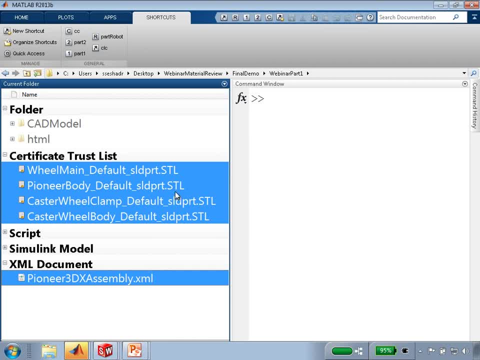 You can also prove this simulation proven algorithm in a real robot as shown in video 2 here, where the real robot is doing obstacle avoidance. You can also prove this simulation proven algorithm in a real robot as shown in video 2 here, where the real robot is doing obstacle avoidance. 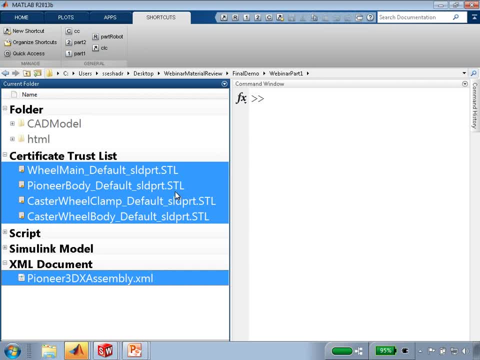 You can also prove this simulation proven algorithm in a real robot as shown in video 2 here, where the real robot is doing obstacle avoidance. You can also prove this simulation proven algorithm in a real robot as shown in video 2 here, where the real robot is doing obstacle avoidance. 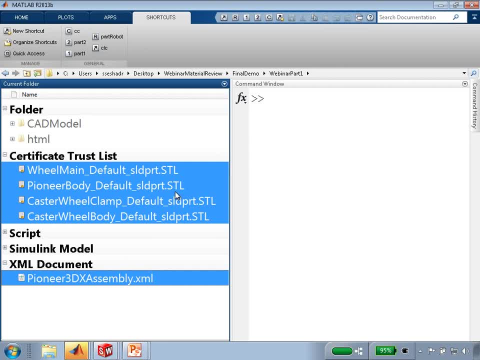 You can also prove this simulation proven algorithm in a real robot as shown in video 2 here, where the real robot is doing obstacle avoidance. You can also prove this simulation proven algorithm in a real robot as shown in video 2 here, where the real robot is doing obstacle avoidance. 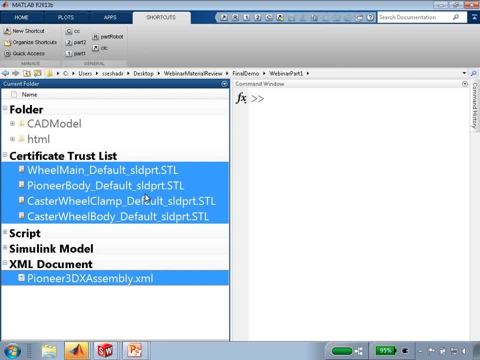 You can also prove this simulation proven algorithm in a real robot as shown in video 2 here, where the real robot is doing obstacle avoidance. You can also prove this simulation proven algorithm in a real robot as shown in video 2 here, where the real robot is doing obstacle avoidance. 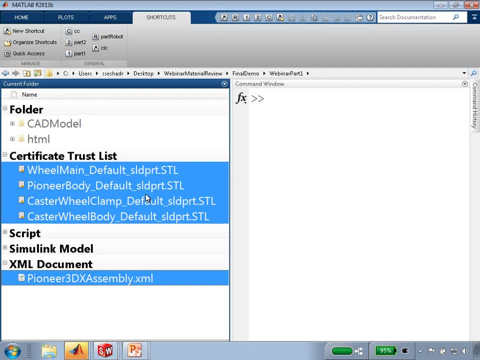 You can also prove this simulation proven algorithm in a real robot as shown in video 2 here, where the real robot is doing obstacle avoidance. You can also prove this simulation proven algorithm in a real robot as shown in video 2 here, where the real robot is doing obstacle avoidance. 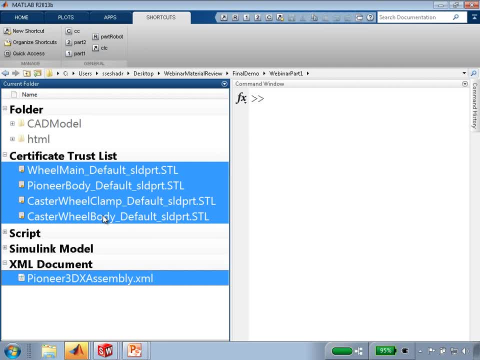 You can also prove this simulation proven algorithm in a real robot as shown in video 2 here, where the real robot is doing obstacle avoidance. You can also prove this simulation proven algorithm in a real robot as shown in video 2 here, where the real robot is doing obstacle avoidance. 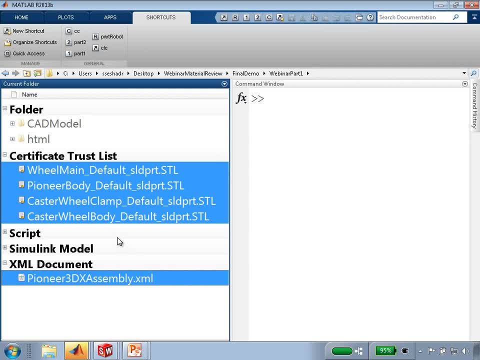 You can also prove this simulation proven algorithm in a real robot as shown in video 2 here, where the real robot is doing obstacle avoidance. You can also prove this simulation proven algorithm in a real robot as shown in video 2 here, where the real robot is doing obstacle avoidance. 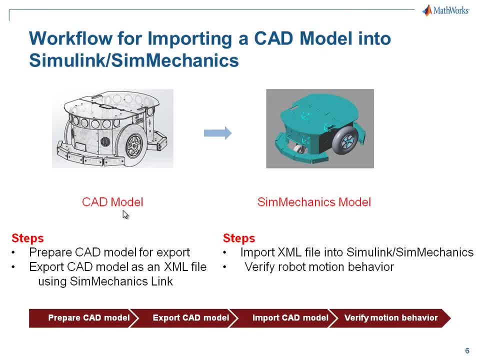 You can also prove this simulation proven algorithm in a real robot as shown in video 2 here, where the real robot is doing obstacle avoidance. You can also prove this simulation proven algorithm in a real robot as shown in video 2 here, where the real robot is doing obstacle avoidance. 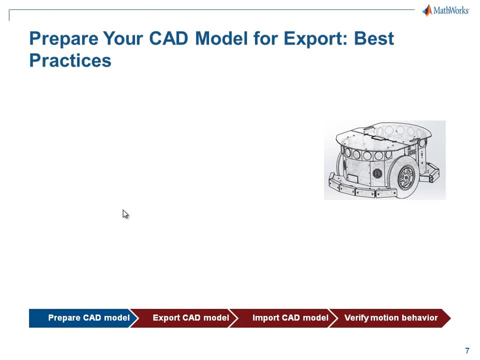 You can also prove this simulation proven algorithm in a real robot as shown in video 2 here, where the real robot is doing obstacle avoidance. You can also prove this simulation proven algorithm in a real robot as shown in video 2 here, where the real robot is doing obstacle avoidance. 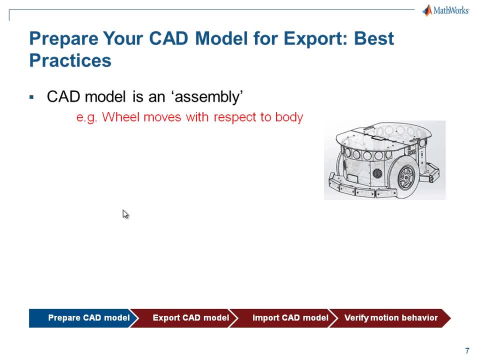 You can also prove this simulation, proven algorithm, in a real robot, as shown in video 2 here, where the real robot is doing obstacle avoidance. First, make sure that the CAD model is an assembly with the right mates describing the relationship between various moving components. 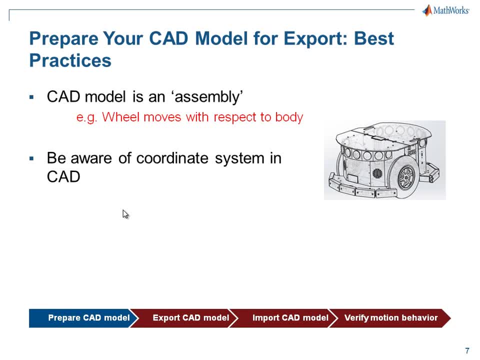 Make note of the coordinate geometry that the CAD model is using. This will come in handy to figure out the gravity vector direction for the simulation. SimMechanics link does have some limitations when it comes to translating some mates. Please consult the documentation if a particular mate has not. 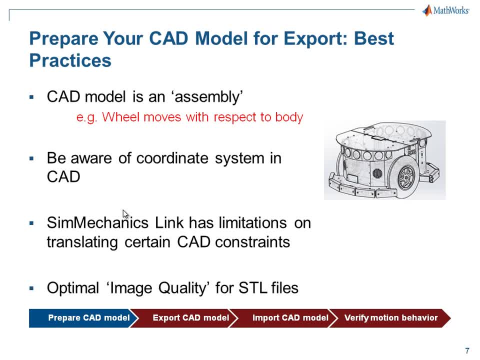 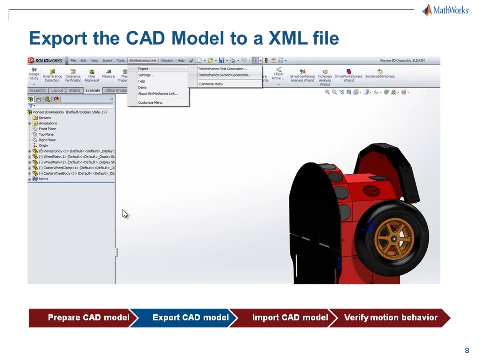 translated correctly. Finally, to reduce the risk of slow simulation or large files generated during export control, the resolution of the parts graphics using the image quality parameter. Exporting CAD model is done from directly in SOLIDWORKS using an add-on software called SimMechanics. link. 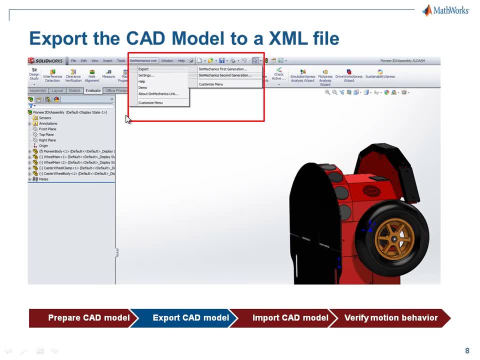 Once you install the software you will see a SimMechanics link menu. You can click on Export SimMechanics Second Generation and then go about translating the file from the CAD model to an XML file. The SimMechanics link add-on can be downloaded from the MathWorks. 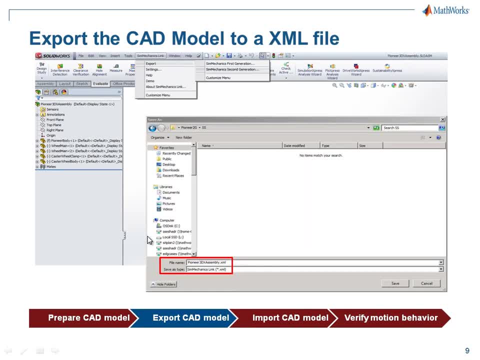 website at this particular link. Once you do that, you can give an appropriate file name and then hit Save, and it would be saved in a given path. You will also get a pop-up message which tells you that the generation was complete. Now that the export is complete, let's. 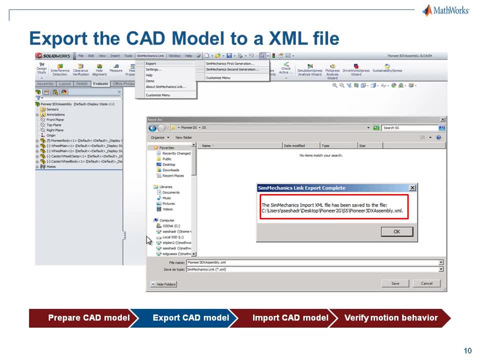 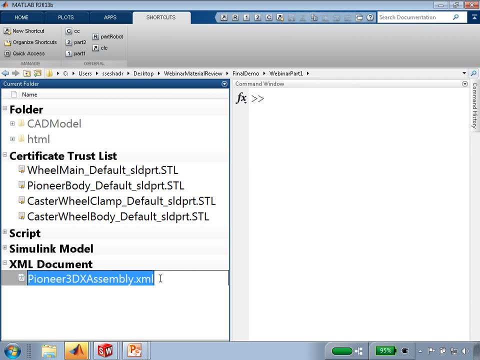 see how to import this XML file into SimMechanics. For this I'm going to use the XML file, I'm going to go back to MATLAB. So once you have this XML file, you can issue a simple command called smimport. 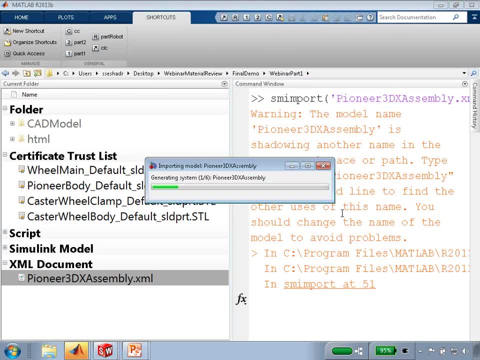 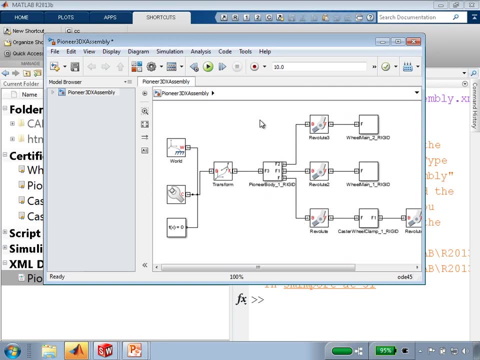 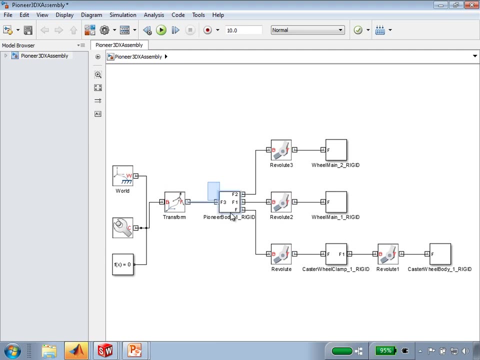 and then provide the XML file name and then hit Enter. This would automatically bring a model which is translated using the XML file. Let's take a look at this model a little bit. You can see that there is a robot body block And there are some wheels and the robot. 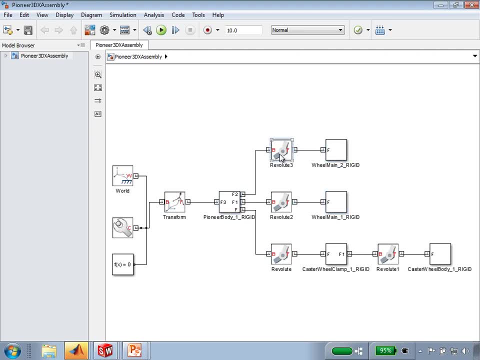 is attached to the wheel using a block called Revolute Joint. This makes sense because the wheel can move with respect to the body only through its rotation about the axle, at least in an ideal sense. You can see a similar pattern with the caster wheel clamp. 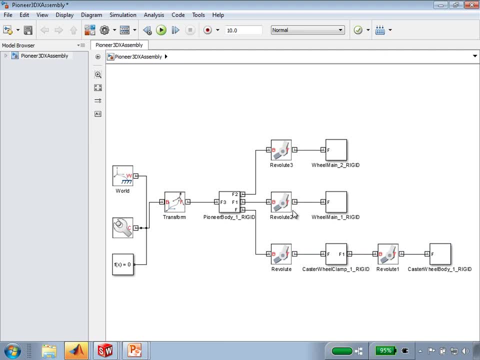 and the caster wheel body. However, we can also realize that this is going to be is going to become a bit cumbersome to identify relationships like this for a complex machine. This is where the built-in 3D viewer of SimMechanics 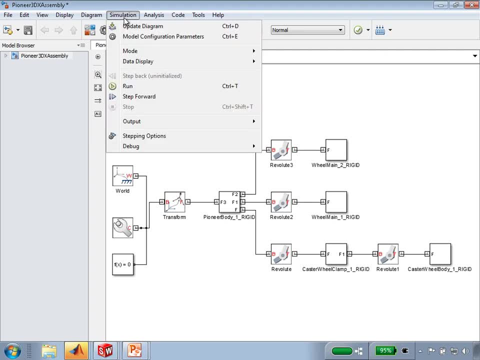 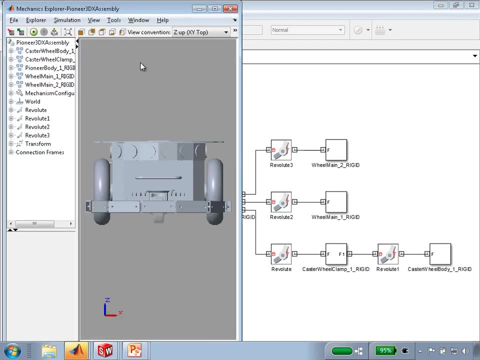 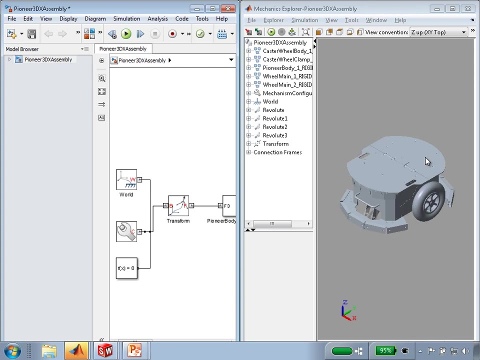 comes in handy. Let us update this model by going to Simulation Update Diagram, And this is going to bring up a window called Mechanics Explorer, which is the built-in 3D viewer from SimMechanics. Here is where the STL files that were generated during the export. 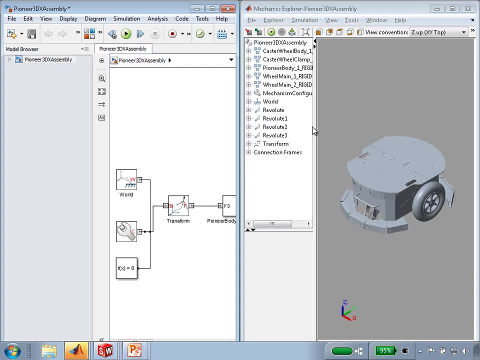 are automatically being used. You can click on the various subsystems in the Explorer window and see the associated coordinate frames attached to these subsystems. Here I'd like to introduce the concept of physical modeling, Although we are looking at a model here which 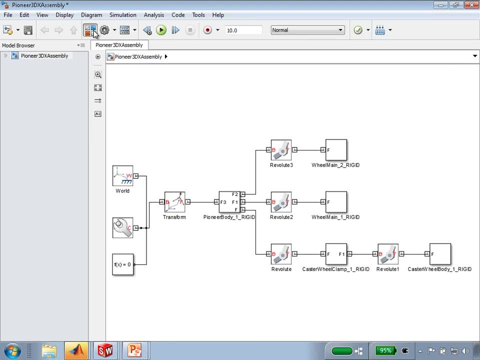 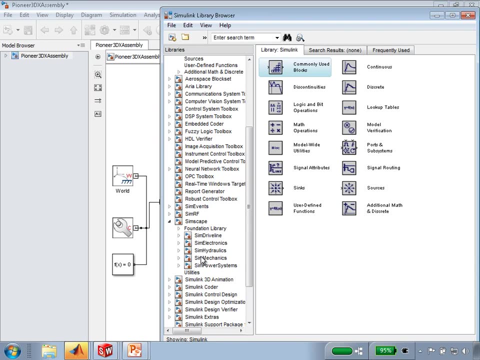 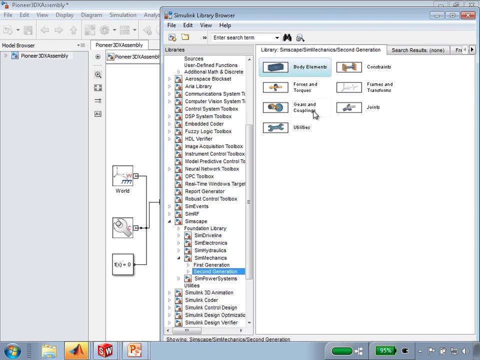 is in the Simulink editor. all the blocks here belong to a subsystem called SimMechanics. SimMechanics is a block set of Simscape which is the physical modeling suit here. so you can see a number of blocks here called body gears and everything which relates to mechanical systems, physical 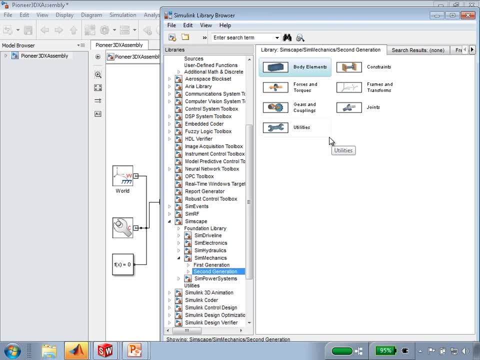 modeling helps you model multiple domains such as electrical, hydraulic and mechanical system in the same environment, as you can see here. let me show you a few examples. here you can see the simscape library. if you go under sim electronics, for example, under passive devices, you can see different components. 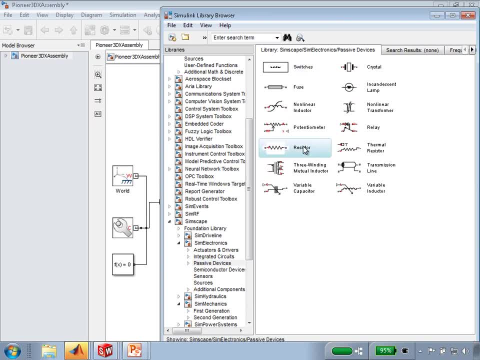 like switches, resistors, etc. physical modeling is just like simulink when it comes to simulating systems based on first principle equations. in physical modeling, however, you have more flexible parameters to tweak and attain different levels of fidelity that you want without having to rewrite all the first. 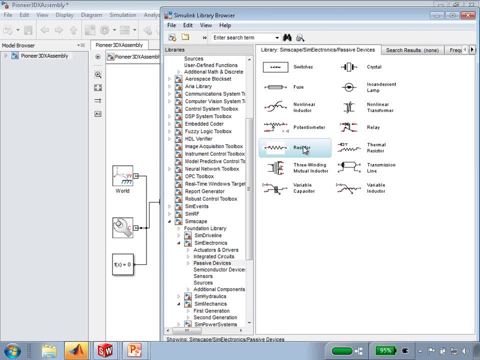 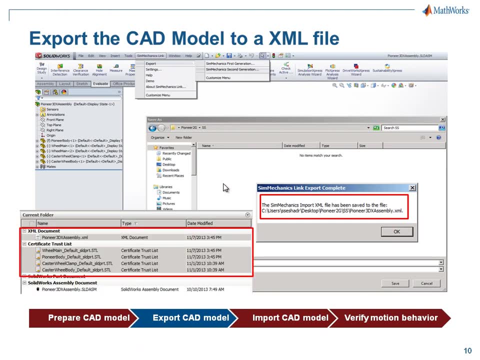 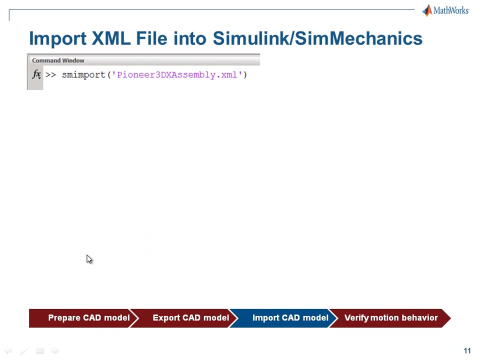 principle equations with different sets of assumptions. now let's go back to the presentation and do a small recap. so we saw that these are the bunch of files that were generated using the export. in order to import it into sim mechanics, we issue a simple command called SM import, which automatically. 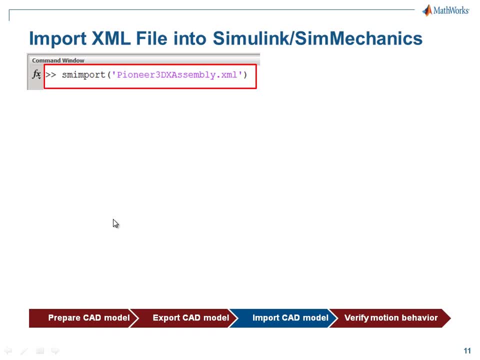 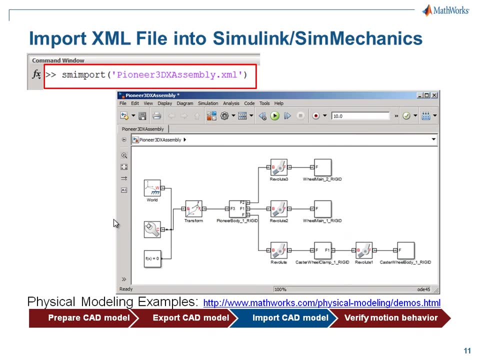 translates the XML file into similar sim mechanics model. we also discussed about physical modeling and you can find some really interesting examples at this link. we also discussed the also discussed the parts in the imported model, such as the robot body and how the wheels are attached to the robot body. Updating the model brings up a window called. 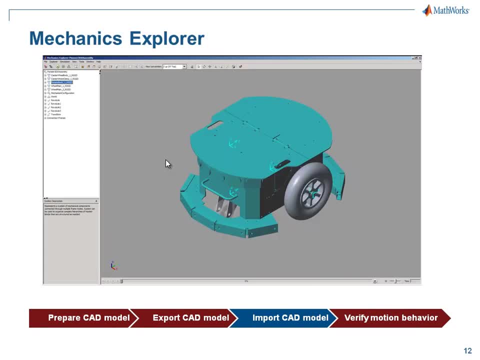 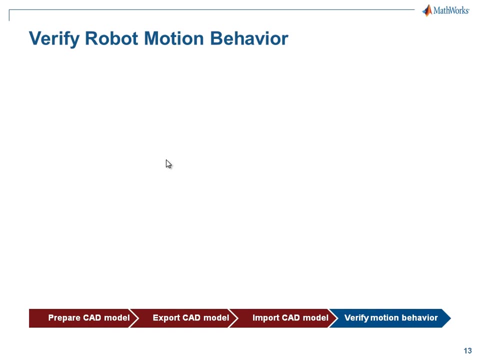 Mechanics Explorer. This is the built-in 3d viewer for the machine in the model. Here is where the generated STL files are automatically being used. Now that we have successfully imported the model, our next task would be to verify the robot motion behavior, In other words, test the robot for mathematical correctness by 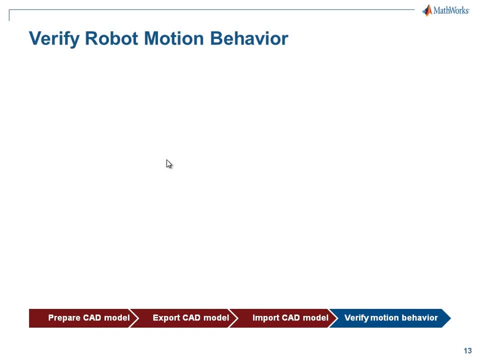 creating some test cases. Here are a few test cases that will help us cover the basic robot motion behavior. Test 1 is an unactuated test to see what the robot does under just the force of gravity. Test 2 adds a simple actuation to see. 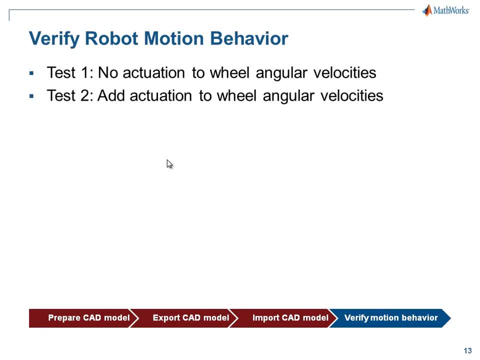 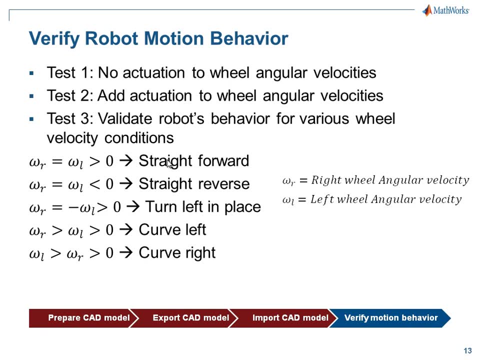 what the robot does under actuation. We test for specific velocity conditions in test 3., Which are basically here. you have the right and left wheel angular velocities and you can test for different conditions to see when the robot moves straight and when the robot turns etc. I'm going to switch to MATLAB to show. 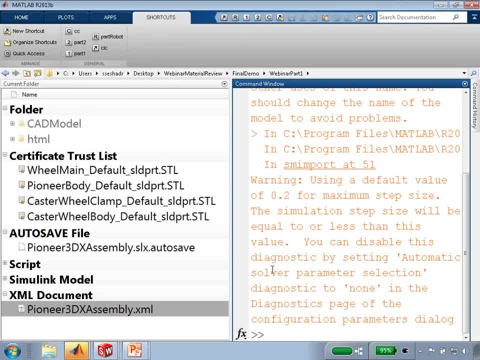 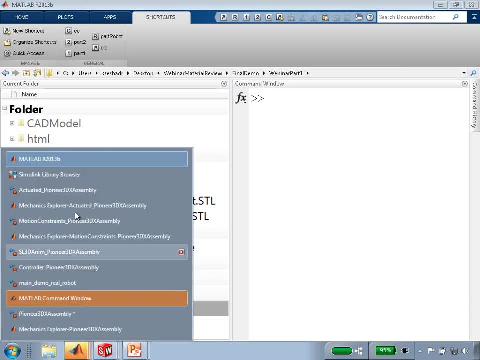 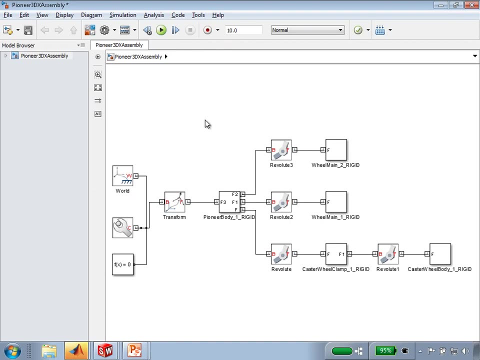 you how these tests are done. So once you go back to MATLAB, let me bring up the model that we are working with. Here is the model which was got as the result of the import. What we want to do is just hit the play button for this particular model and see. 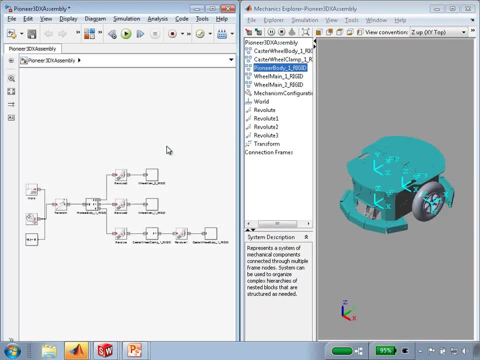 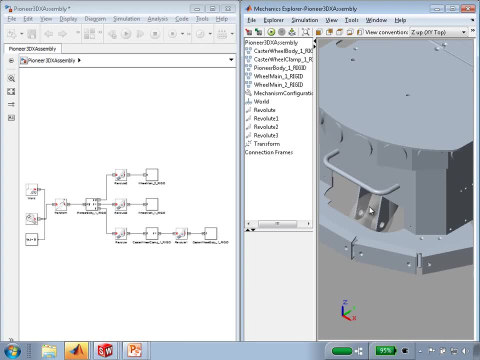 what it does under gravity. So I just want to bring the model and the animation side-by-side Here. if you see, the caster wheel is actually oscillating. This is not expected behavior, because under gravity the robot should just stay put. Let's take a look at this particular block called the mechanism configuration. 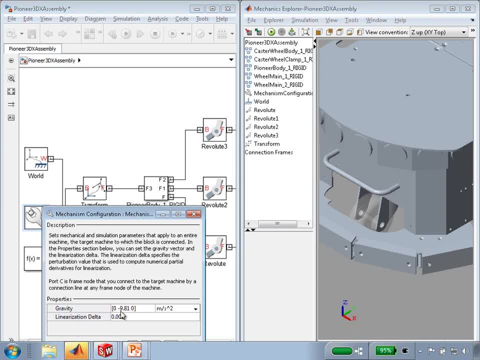 block and look at the gravity vector. The gravity here is in the negative y direction. However, it should be in the negative c direction here. This is where knowing where the robot came from and what is the coordinate system it lived in in the CAD model makes sense. 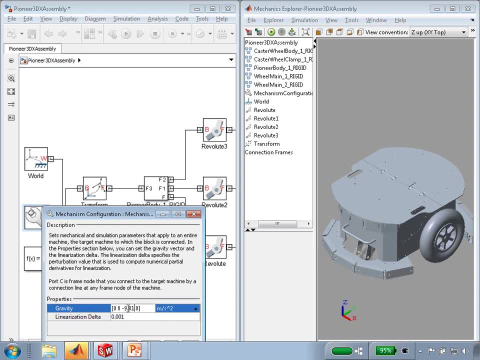 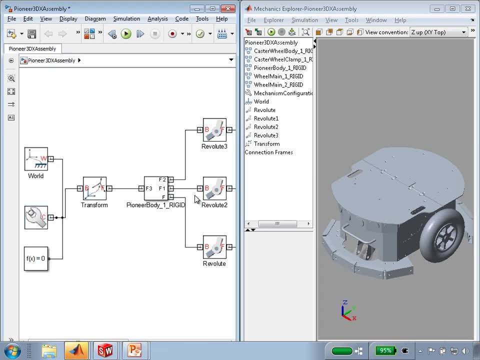 So if we just change this to 00-9.81, so that it's in negative z direction, and apply the changes 0-9.81.. 0-9.81.. 0-9.81.. 0-9.81.. 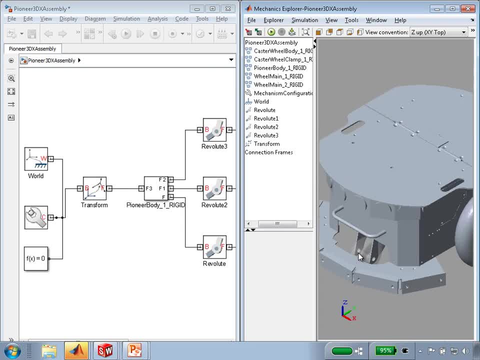 0-9.81.. 0-9.81.. 0-9.81.. Again, let's see if the caster wheel still moves. Now we see that the caster wheel doesn't move, and this is the expected behavior. This is test one. 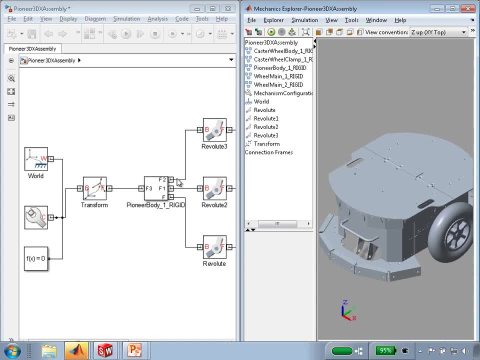 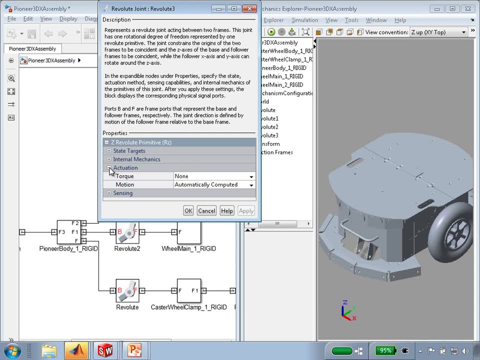 Now let us add actuation, which is our second test. Actuation can be added by accessing the joint blocks and the actuation parameters. here We are going to provide motion as input and we are going to automatically compute the torque that is required to get that motion. 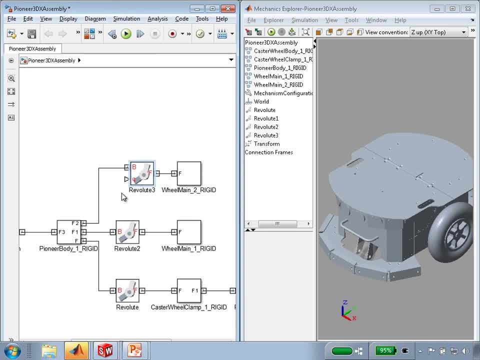 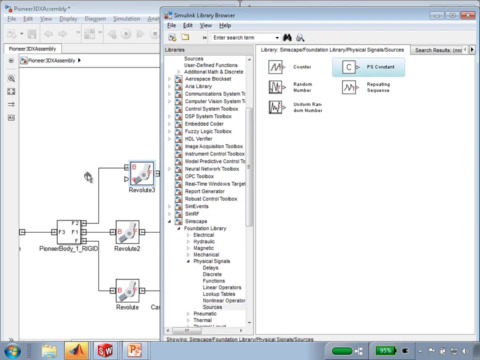 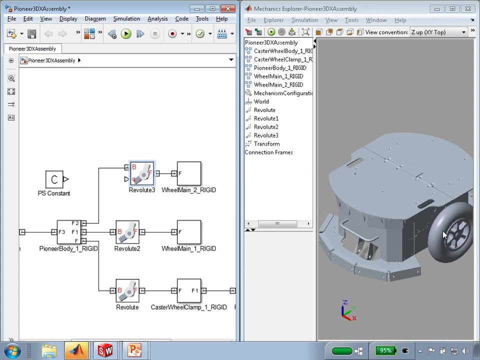 When this is chosen, an extra signal port appears here for you to give the input. The revolute joint takes the angular position as input. So let's go back to Simscape and let us get a source which is a constant. Now, if we feed in this constant to the revolute joint, this is going to make the robot move. 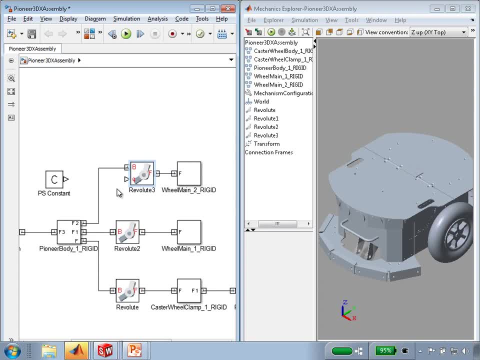 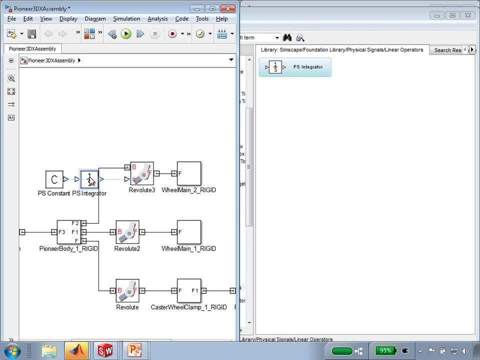 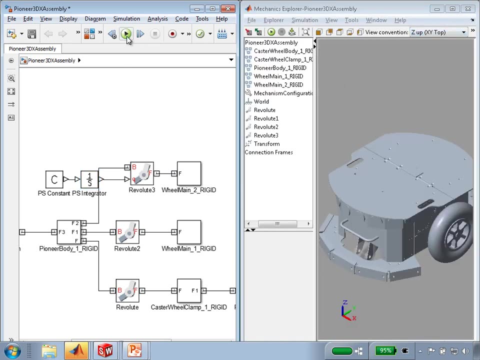 the wheel once, Once and stop, But we want it to rotate at a constant rate. So let's also bring in an integrator which is going to integrate the constant rate and give us a ramp kind of signal for the angle. So if we do this and hit, play and look at what the robot does for this wheel, we see 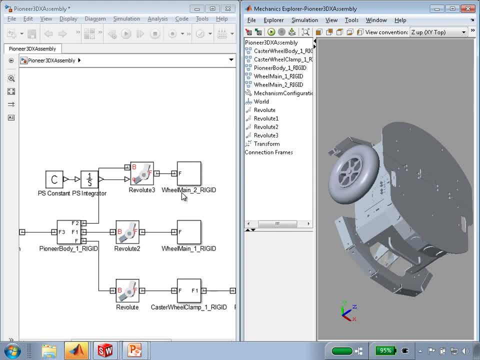 that the wheel moves at a constant rate. Now we can already see that the model is becoming a little cumbersome to handle here. So in order to make it more readable and easier to understand, you can select these blocks together and, let's say, create a subsystem so that and then let's call it right view. 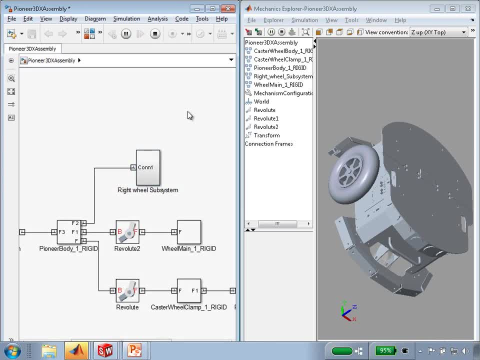 subsystem and then hit play. Now you can see that the robot functionally hasn't changed, but now it's easier for us to maintain the system. And here is where the change has occurred. Similarly, I can do this for the other wheel as well. 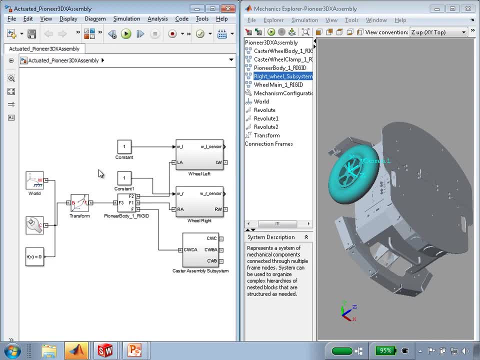 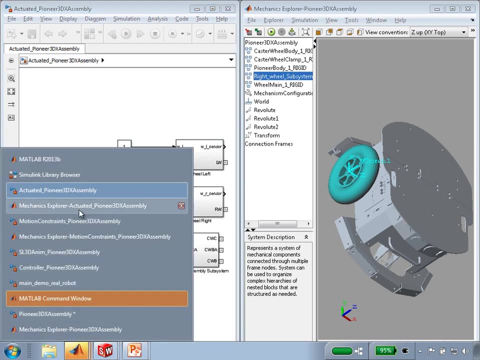 And I'm going to bring up the model where I've already done that. So here is the model where I have constants fed in as input to omega L and omega R of the wheel, And these are the left and right subsystems. Let me also bring in the animation with respect to this. 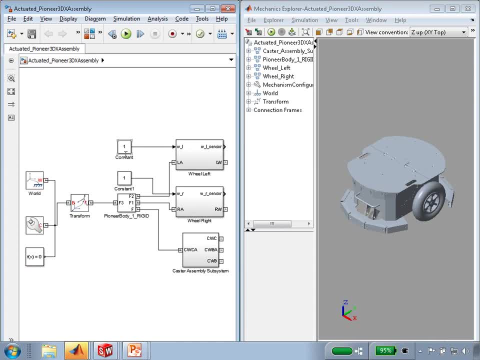 Now, if I simulate, I'm expecting the robot to actually move in a straight line because I'm feeding it constant angular velocities here. If I hit play here, I see that the robot actually doesn't move. This is because the CAD model does not possess the information of what the robot should do. 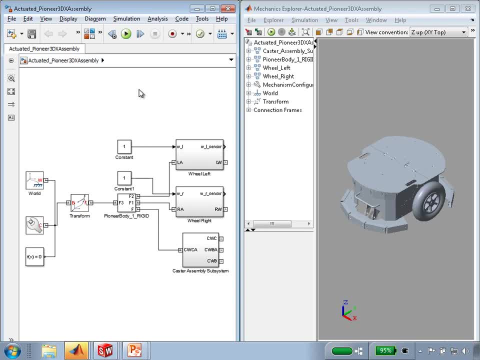 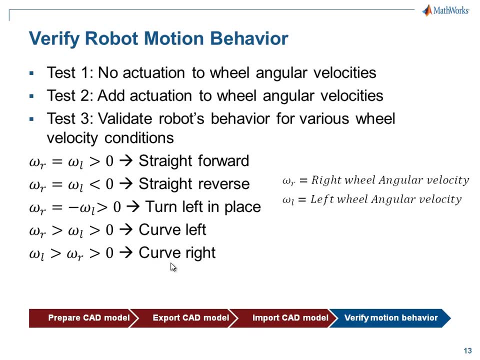 with respect to the world as a frame. Here is where we need to add our own constraints to make the model more detailed. Let me go back to the presentation to do a recap. We just simulated the robot model under gravity and saw that the caster wheel was oscillating. 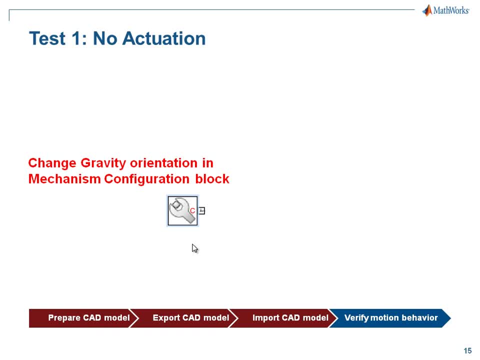 So we can see that the robot is moving in a straight line. So we can see that the robot is moving in a straight line. So we can see that the robot is moving in a straight line. We checked the gravity orientation in the mechanism configuration block and we changed. 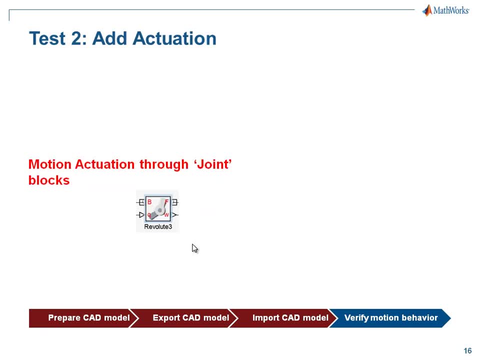 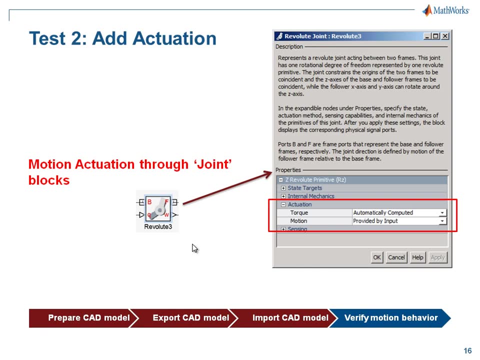 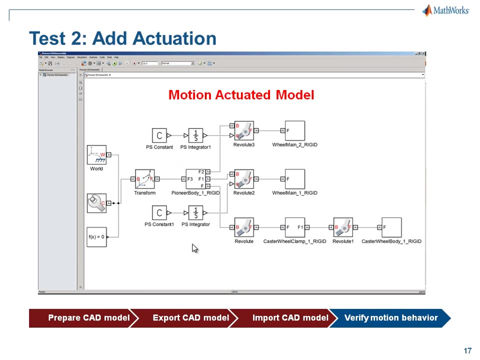 it as we wanted it to. We implemented the motion actuation by providing input to the motion and automatically computing the torque. When this is chosen, an extra signal port appears to feed in this value. This is how our motion actuated model looks like. 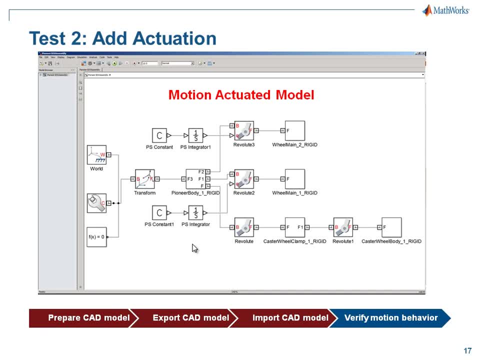 The revolute joint takes an angular position, so in order to keep rotating it at a constant rate, we feed a constant through an integrator to keep the wheels in motion. Essentially, we are specifying the constant angular velocity for the joints here. However, since the robot does not move anywhere, we need to model additional constraints. 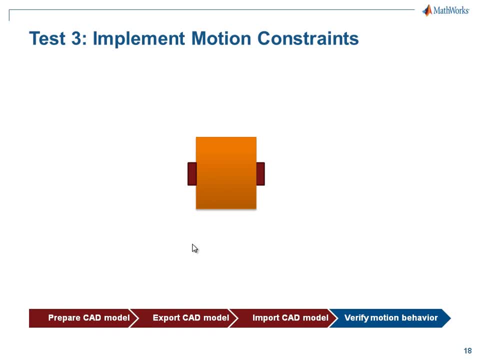 In order to understand the missing constraints, let us take a look at mathematically how the robot moves. Let us consider that the red dot is the center of mass of the robot, The brown parts are the wheels and the orange part is the body of the robot, and this is 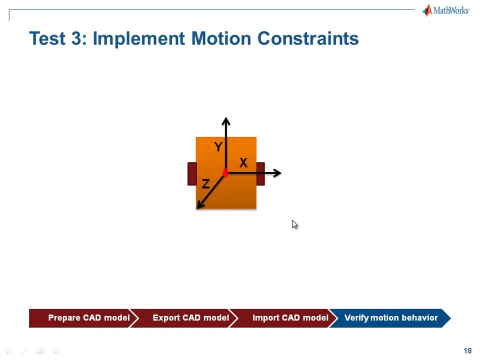 the top view of the robot. Now, the robot's pose can be defined entirely by knowing its position in the XY frame, which is PX and PY. Also, the robot could rotate, and let us suppose that this rotation angle is theta. Now the actuation inputs to the robot are the individual wheel, angular velocities, omega. 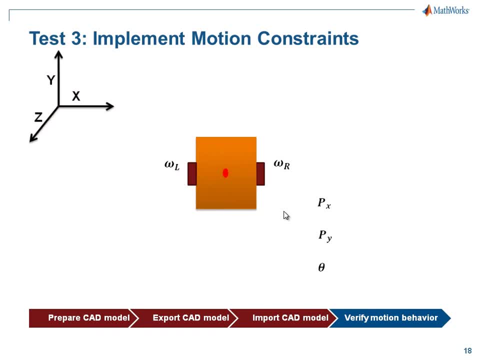 omega and omega. The rotation angle is theta. This is the position for the robot, which is PX, PY and theta. Let us see how we can get from omega L and omega R to the pose of the robot, which is PX, PY and theta. 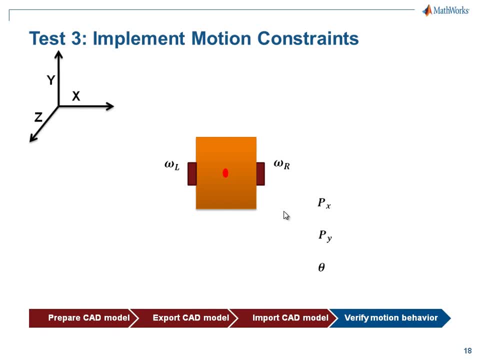 The individual wheel angular velocities. omega L and omega R correspond to a linear velocity of VL and VR. Now the linear velocity of the center of mass of the robot, V, will be the average of these two velocities, When the velocities are not equal to each other. 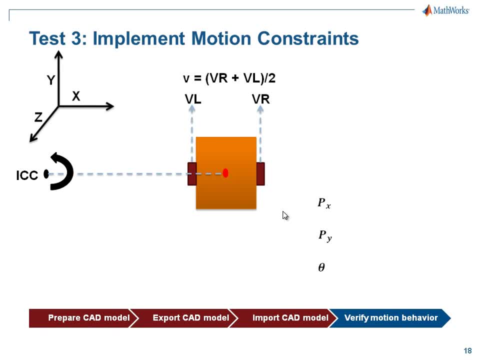 you can imagine that the robot will rotate about an instantaneous center of curvature. This rotation rate can be calculated as shown here, which relates the wheel linear velocities and the track width of the robot, which is the distance between the two wheels. From this, the angle of the center of mass with respect to the center, namely theta, can also be got. 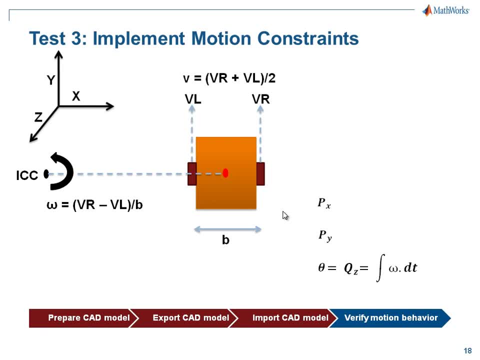 Using this, we can define the robot position in x and y directions, namely px and py, and the robot hitting theta that determines the planar motion of the robot. These parameters can then be fed to a planar joint block to drive the robot center of mass with respect to the whirl frame. 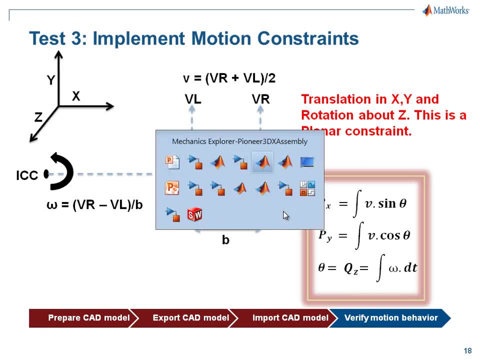 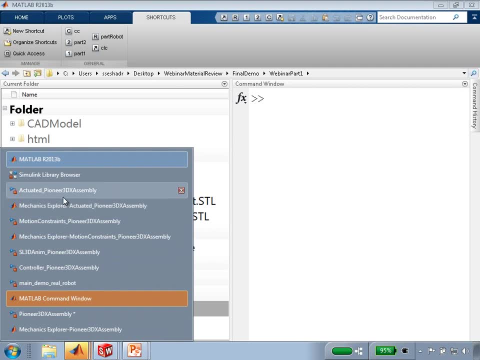 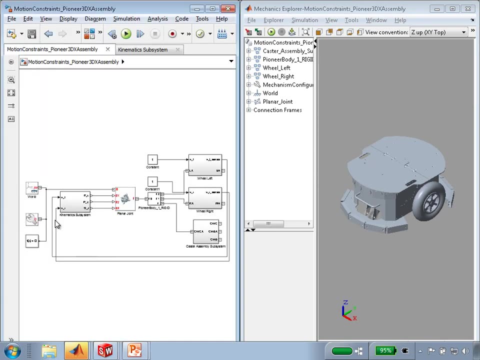 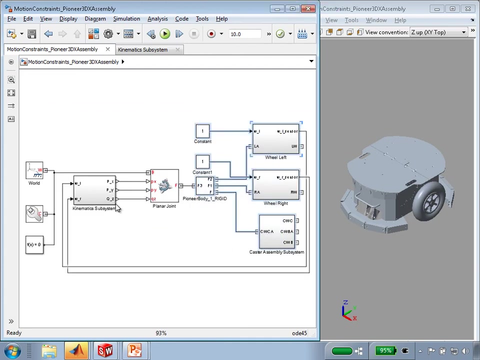 Let me bring up a model where we have already done this. So I'm going to bring up a model where we have already implemented the motion control. So I'm going to bring up a model where we have already implemented the motion control. So here, this is the same as what we had initially. 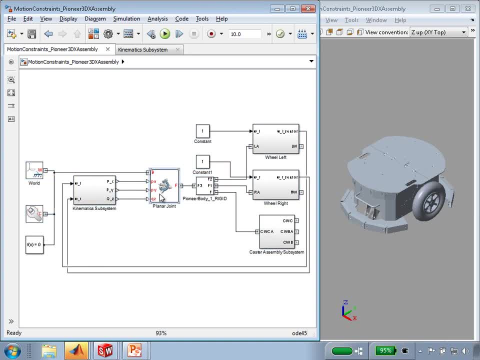 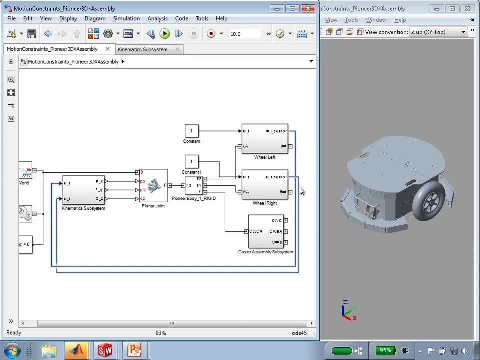 We have two extra blocks here, which is the kinematic subsystem and the planar joint. Essentially, we are sensing the wheel angular velocities and then feeding it to a subsystem. Using that, we are actually calculating px, py and qz, which is theta. 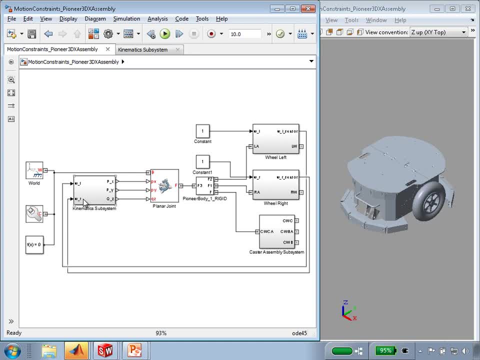 These are the planar parameters of the robot. This defines the relationship between the world and the robot body itself. In order to make this evident, we are using a planar joint block which relates the world and the robot body, and feeding these parameters that we got by calculating. 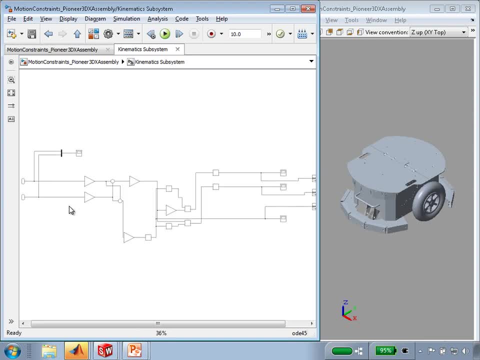 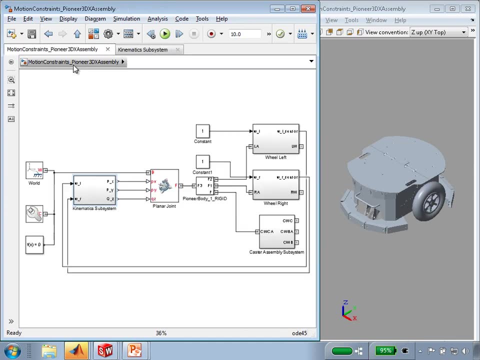 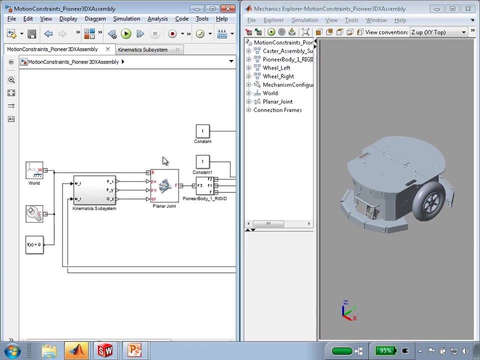 calculating using the equations that we just described. These equations are here laid out in a graphical form. You could also write a MATLAB function to do this. So once we do this, where we have actually showed how the robot should move with respect to the world, 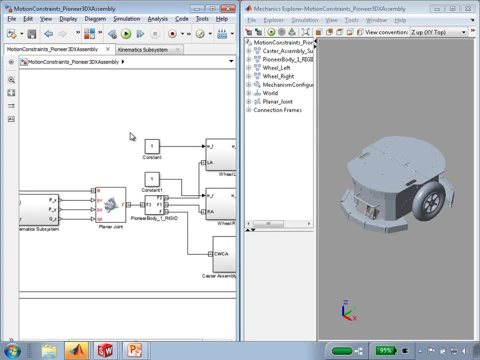 we expect the robot to move in a manner that we think. So when we give omega l and omega r equal to each other, we are expecting the robot to move in a state. Let's see if it does that. So when I hit the play button, the robot actually. 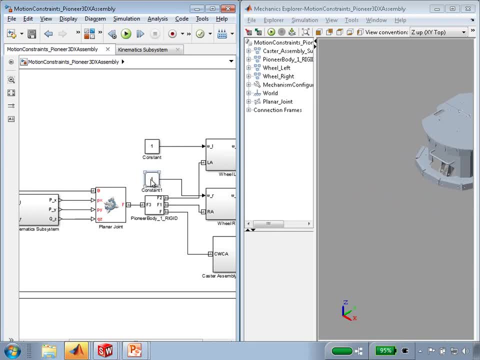 moves in a straight line, which makes sense. Now let's say my omega r is negative of omega l. For this, I'm expecting the robot to rotate about its center of mass. To see this better, I'm going to go to the top view. 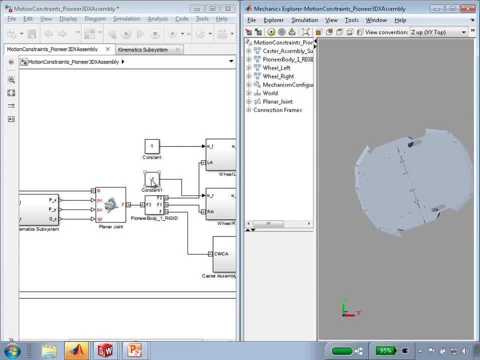 and see that the robot actually moves like this. Now let's make omega r in the same direction as omega l, but of a different magnitude. Now I'm expecting the robot to move in an arc, in some sort of a circle, which I can see that the robot actually does. 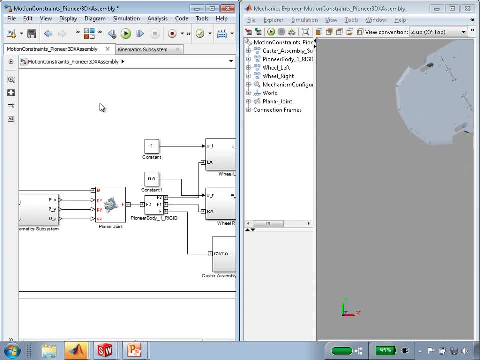 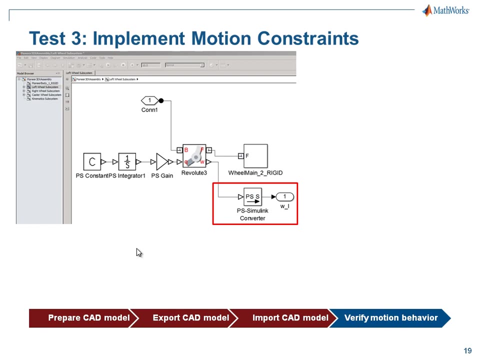 So now we have actually tested one, two and three, the three conditions that we are talking about when we were talking about verifying robot motion behavior. Let's get back to the presentation. This is how our motion actuated model looks like. First we sense the individual wheel angular velocities. 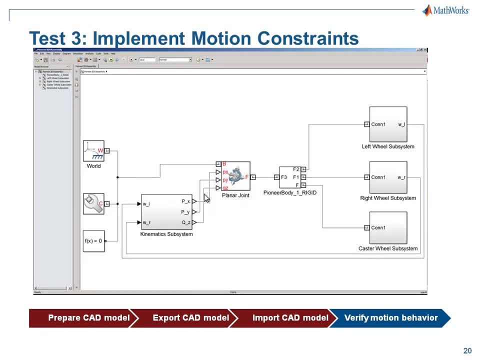 omega l and omega r, And then we implement the equations explained earlier in this kinematic subsystem and then feed it to the planar joint block. This is inside the subsystem that calculates the planar parameters of the robot, which is laid out in a graphical format. 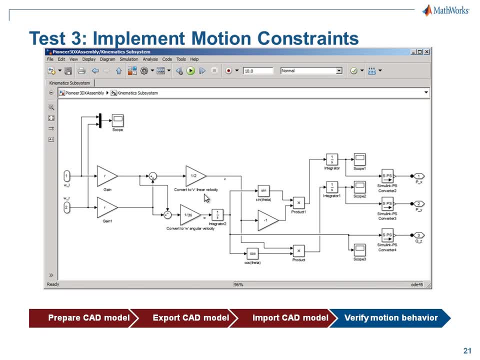 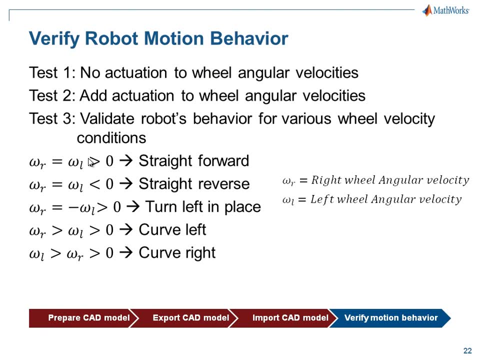 There are multiple ways to do this. You could also use a MATLAB function. Finally, we have now verified the robot motion behavior for various velocity conditions. We tested it for no angular velocity of wheels And no actuation, And we saw that the robot actually doesn't move. 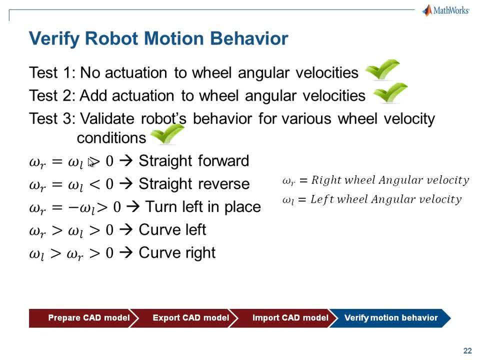 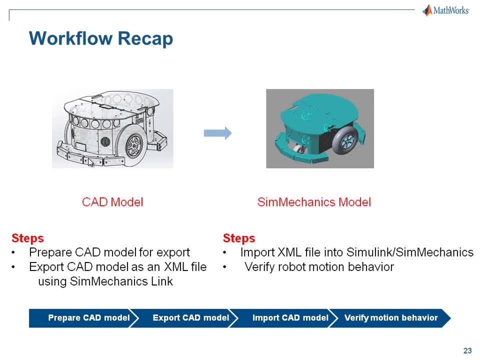 when we actuate the wheels, And then we implemented motion constraints and checked the different angular velocities. To recap the workflow: we started with the CAD model, We then exported it to an XML file and then imported the XML file into Simulink- SimMechanics. 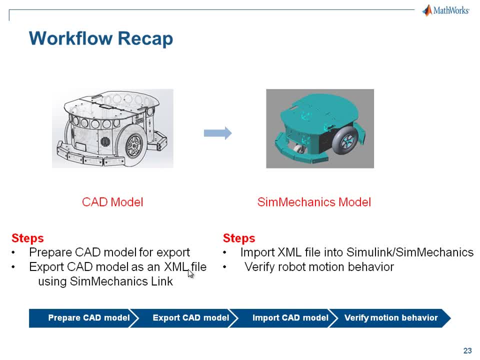 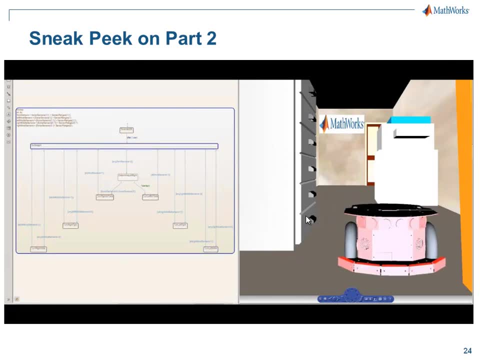 using the SM import command. And finally, we have the robot behavior tested for various test cases. This is the end of first part of the two-part webinar. In the second part we are going to see how to make the robot interact with an external environment. 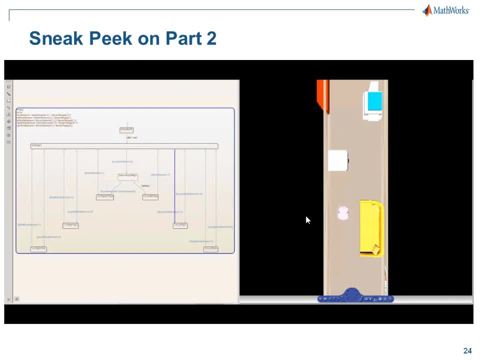 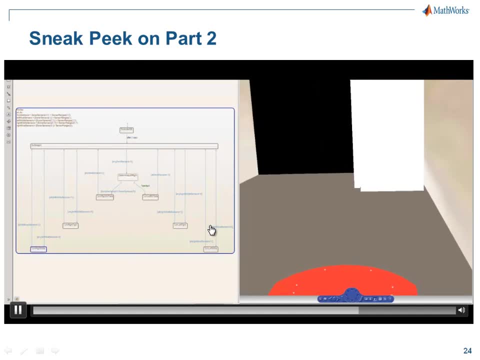 using Simulink 3D animation. as shown in this video, We are going to test collision avoidance algorithm developed using state flow on the left-hand side here And see the robot move and interact with a virtual environment on the right-hand side. 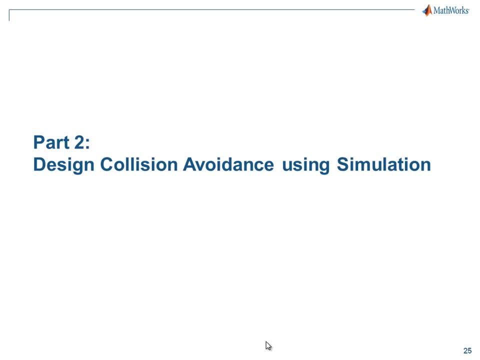 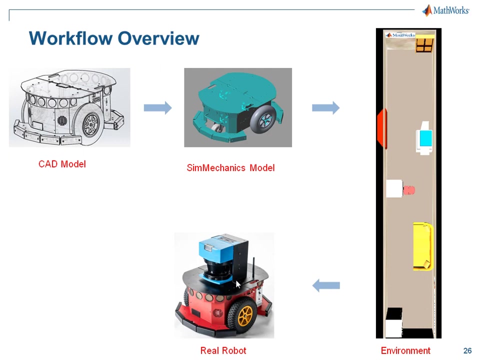 Now that we have a Simulink SimMechanics model of the mobile robot As a result of part one of the webinar series, let's learn how we can use the model to design and test collision avoidance algorithms using simulation. Here is the overview of the overall workflow. 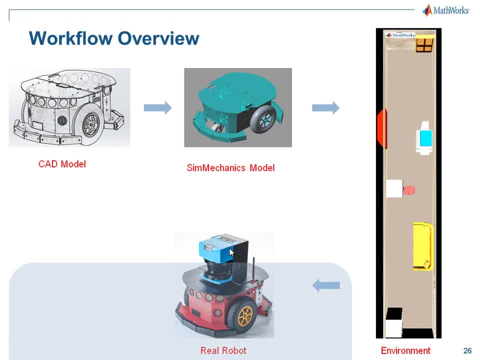 that we are following here today. In part one, we saw how to import the CAD model for a robot into simulation. In part two of the webinar, we are going to use that model developed in part one to design a collision avoidance algorithm and simulate it in a virtual environment. 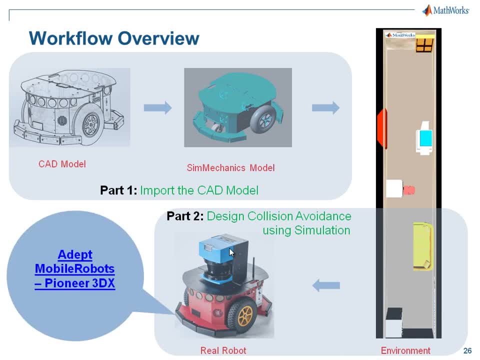 Later we will also be implementing the developed algorithm on a real robot. We used the Pioneer 3DX platform from Adept Mobile Robots for this demo. I will talk about the full capabilities of this robot a little later in this presentation. So let's get to part two of this webinar series. 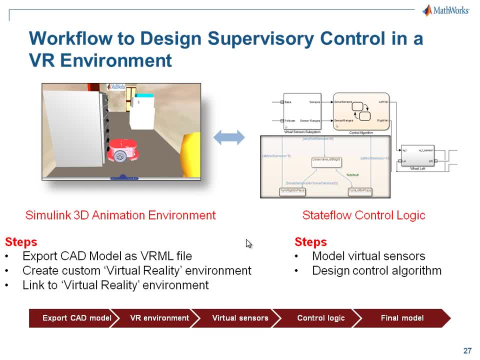 In the second part, as with the first part, we are going to start with the CAD model of the robot. We are going to see how easy it is for making the CAD model interact with the virtual reality environment and how easy it is to design control logic for the robot. 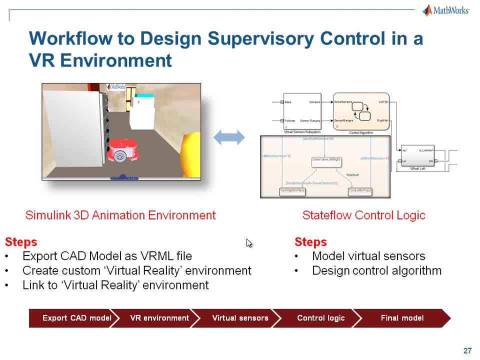 As with the first part, we start with the CAD model. We export this to a standard 3D modeling format called VRML. Later we create a custom virtual world where the robot can actually live in. Finally, we link the 3D animation to the existing dynamic model. 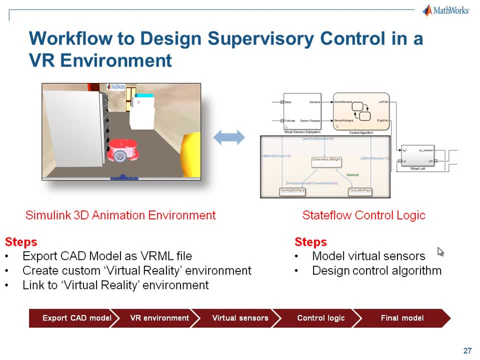 which is the result of part one of the webinar. Then we go on to create the control logic part, where we first talk about modeling sensors virtually and then show an example of how easily one can design supervisory controls using Stateflow. Now let's take a look at the CAD model. 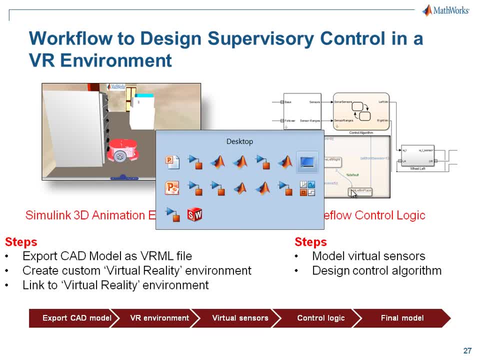 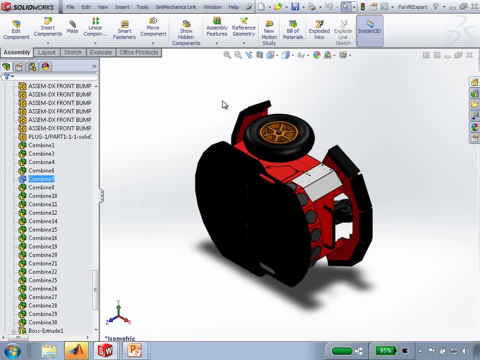 that we are going to use today. So I'm going to switch to SOLIDWORKS again. So for virtual reality file export, we need the CAD model. We are going to use the CAD model to be an assembly, as it was with the part one as well. 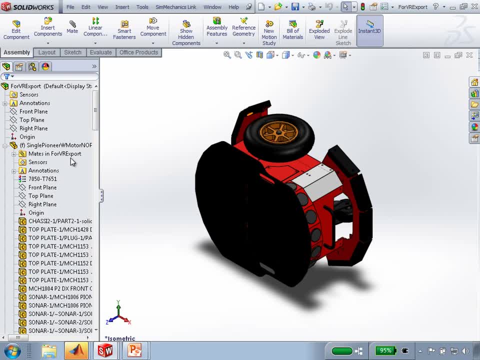 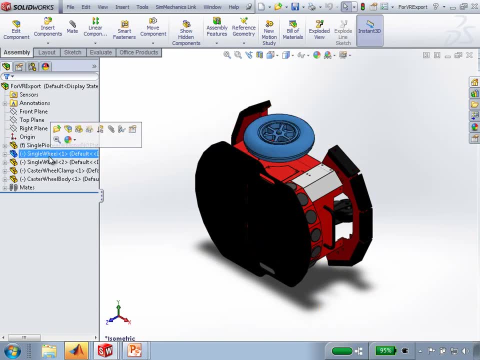 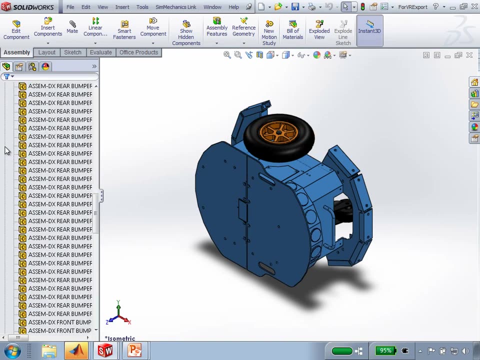 This is very important because the CAD model can have components which can move with respect to each other. As with here, there is the body and there is the wheel, and the wheel can move with respect to the body. Apart from this, the CAD model could have multiple features. 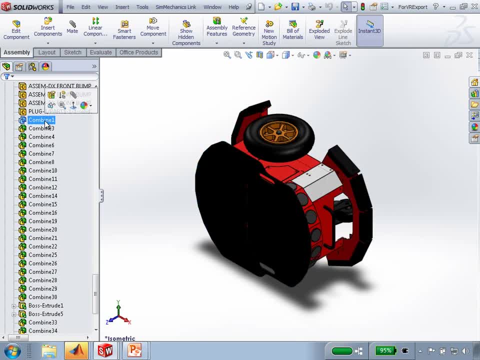 which are multi-body features, and it will be useful for you to combine them with each other so that different parts can be considered a single entity. For example, the wheel spokes and the wheel itself can be considered as the same part, So we need to combine those two features together. 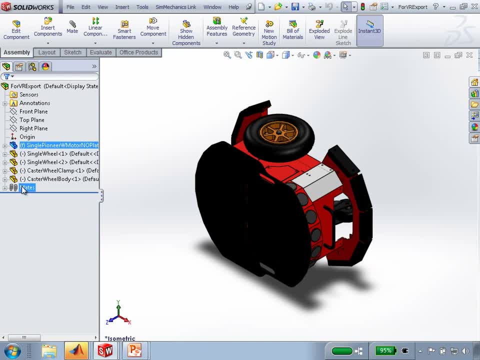 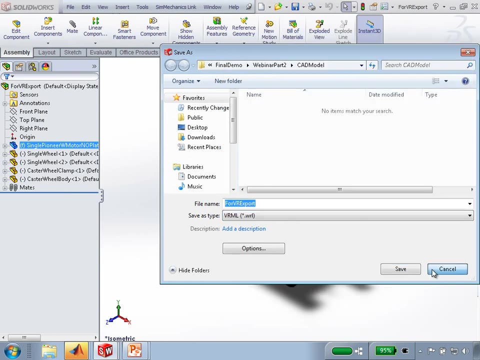 so that they can move as the same as each other. In order to save this as the VRML file, we can go to File Save As and then choose the Save As type as VRML here and give the file name. Once you do that, you can get the VRML file. 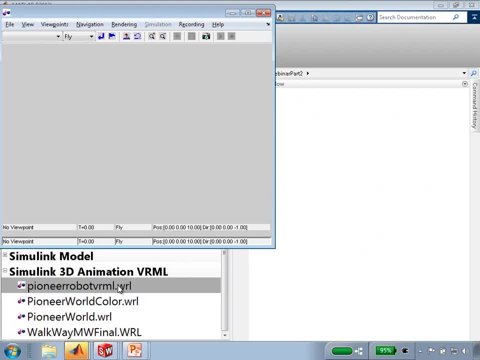 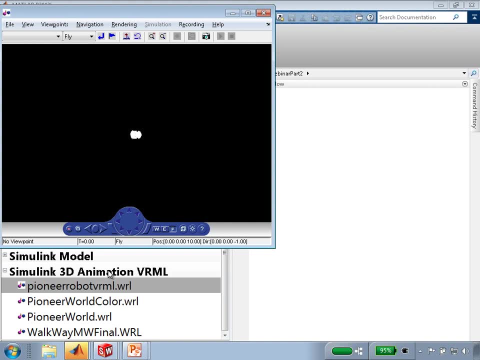 as I'm going to be showing you here. Its extension is WRL and by just double-clicking on the VRML file you can open it. in the built-in 3D viewer that we have, You can zoom in to see how the robot looks like. 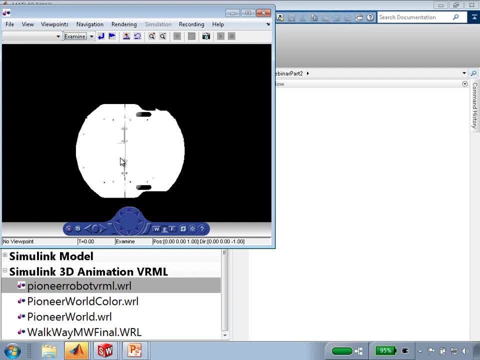 in the 3D animation form and you can examine it to see how it actually looks. here We can see that there is one VRML file here. You could control the resolution of these graphics by setting the image quality parameter appropriately in SOLIDWORKS. 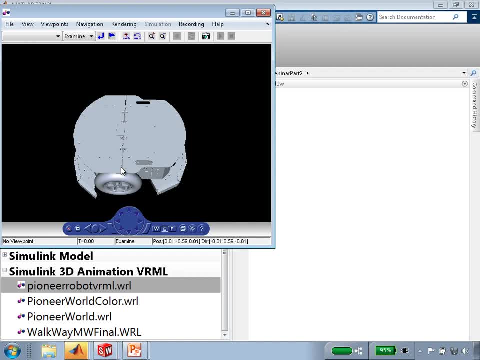 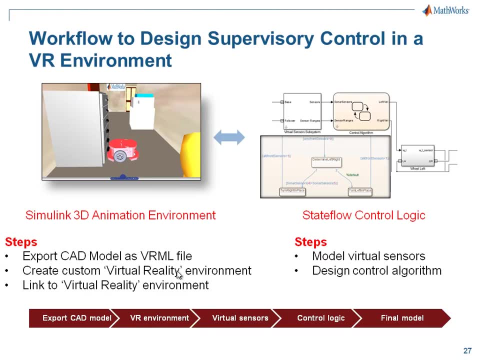 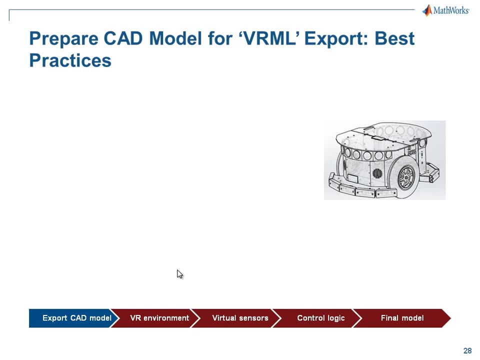 Higher resolution may result in slower simulations because it impacts the rendering speed. Now let's go back to the presentation to do a small recap. So the best practices to prepare CAD model for VRML export are as follows. To reiterate, the CAD model needs to be an assembly. 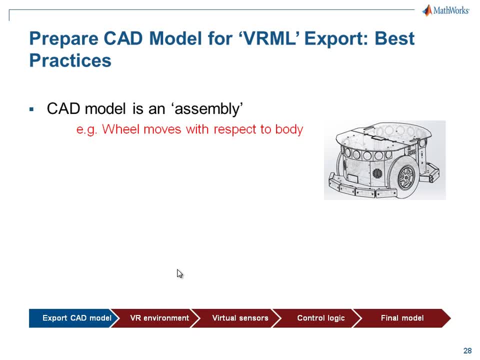 so if a body can move with respect to each other, then we need to specify constraints to show the same thing. If there are multi-body parts, combine them into a single body so that they can move as a single body. Finally, you can tune the image quality parameter. 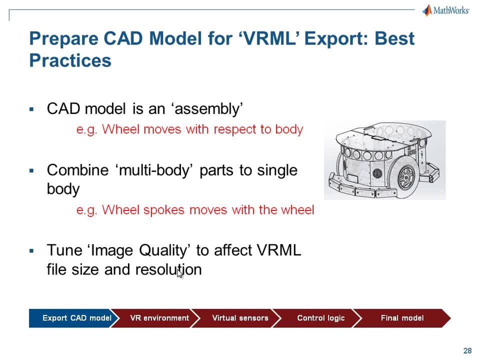 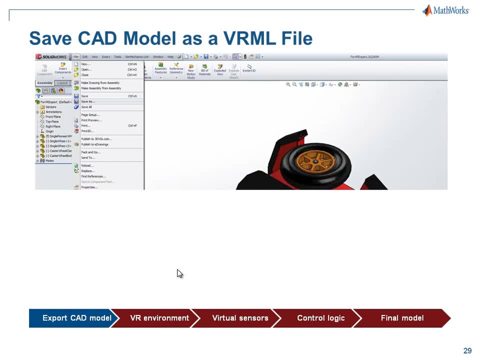 to affect the VRML size and resolution and this affects the simulation speed because it affects the rendering speed. Exporting the CAD model to the VRML format is done from SOLIDWORKS. Just go to File, Save As and then give the appropriate name. 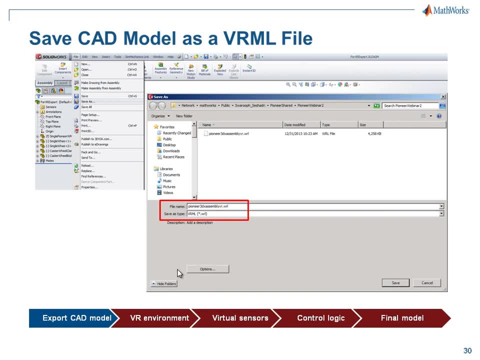 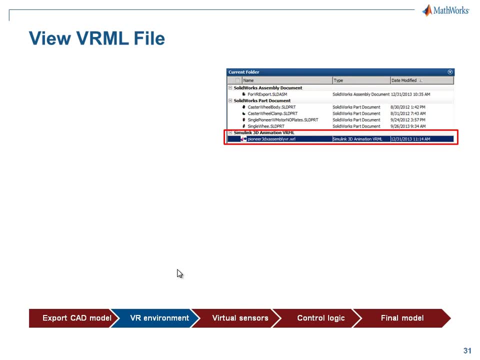 and choose the type as VRML. Once the Save As is complete, you can go to the specified location to take a look at the WRL file. In order to view this in the built-in 3D viewer, double-click on the file name. 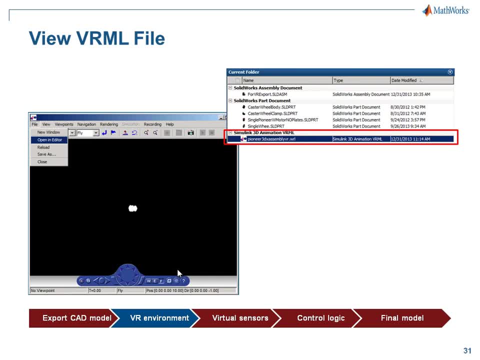 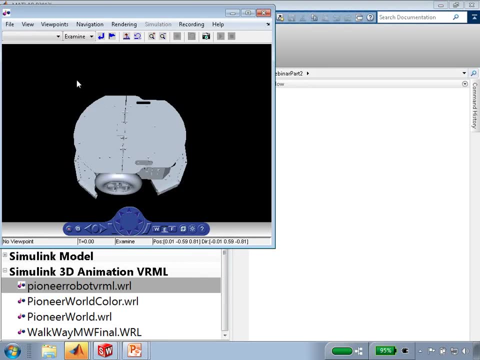 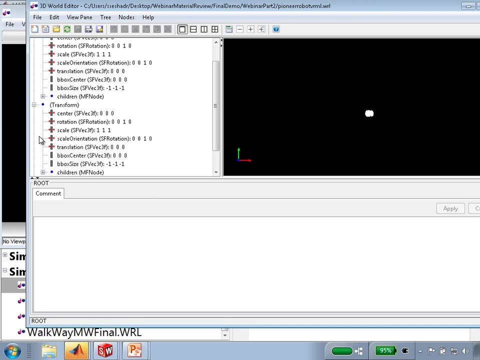 To view the file structure, go to File Open in Editor. Let's go back to MATLAB and see that, So you can just go to File Open in Editor and this will open it up in an editor where you can actually look at the file structure here. 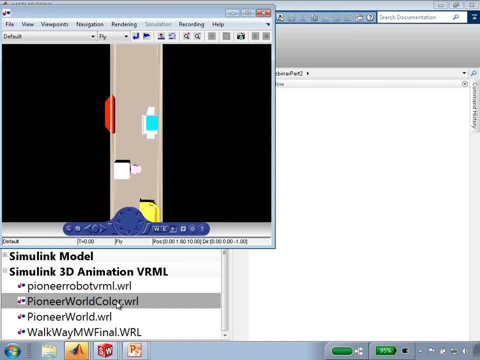 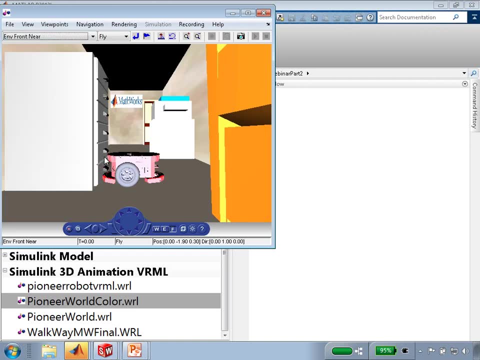 Let me actually show you the final 3D model that we are going to use here today. Here we can see that the robot is actually living in an environment. Since building these custom environments is not the particular focus of this webinar, I will point you to the resources. 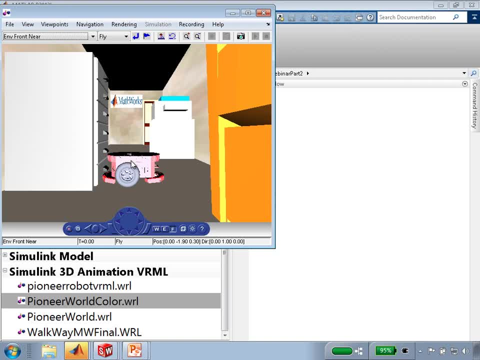 on our website later. that will help you with these kinds of projects, authoring detailed scenes like this. I would like to talk a little bit about simulating 3D animation. 3D animation helps you test algorithms by giving you the capability to interact. 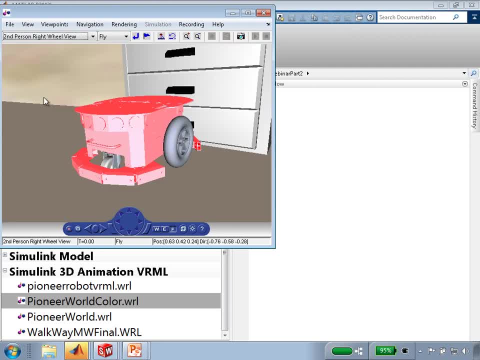 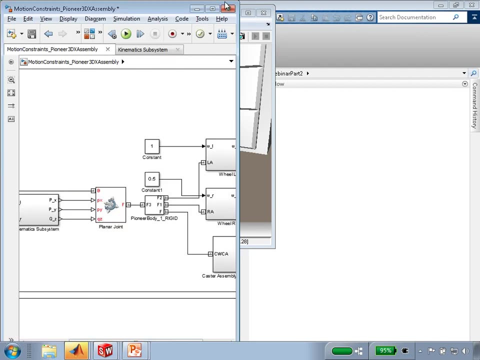 with virtual objects like this here. It also helps you author detailed scenes and helps you visualize dynamic systems in a virtual world. Let me first pull up the model which was the result of part one of the webinar, which is here. So we have the sim mechanics model. 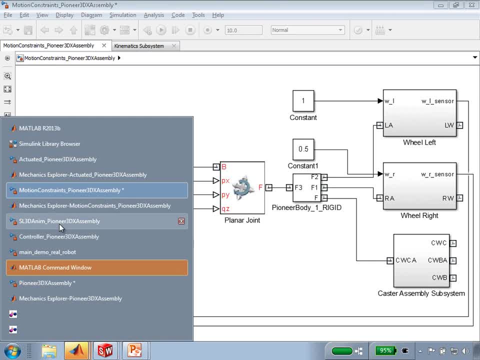 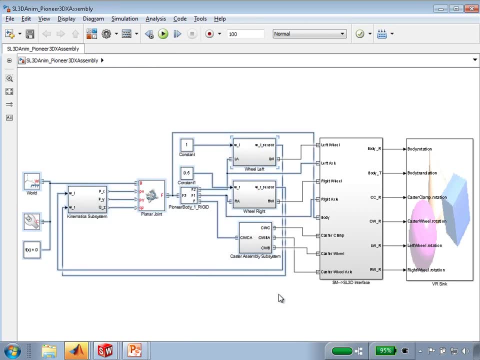 we have the kinematics and everything. Let me pull up the model which links this model to the simulating 3D animation here. So this is the result of part one of the webinar series and these are the two extra blocks that are necessary at this point. 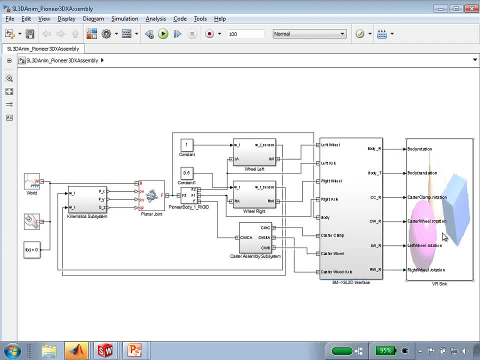 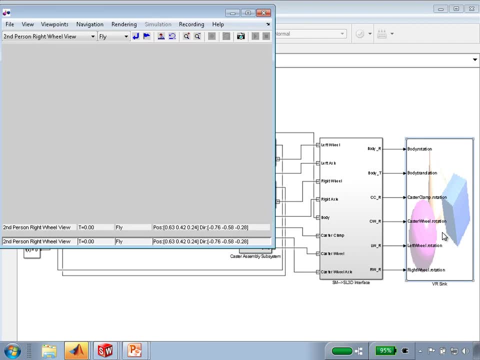 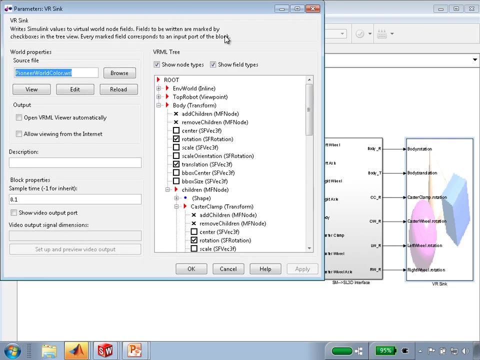 for us to link the two together. First, the VR sync block that gets actuation inputs for the robot animation. By double-clicking the block we can actually see the robot in its environment. Clicking on the block parameters icon here will bring up the VR mask. 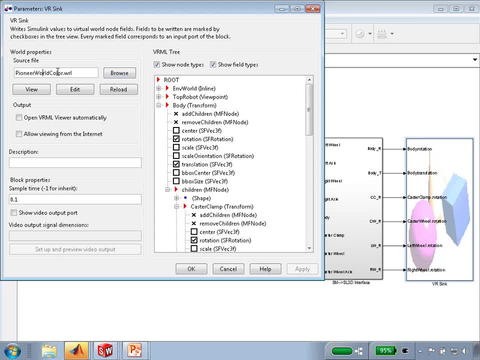 We also specify the actual file that it needs to use here. Apart from this, the VR block itself is inanimate. You need to feed it inputs in order to drive the animation. In this particular example, you have the robot's body and you are providing it the rotation matrix. 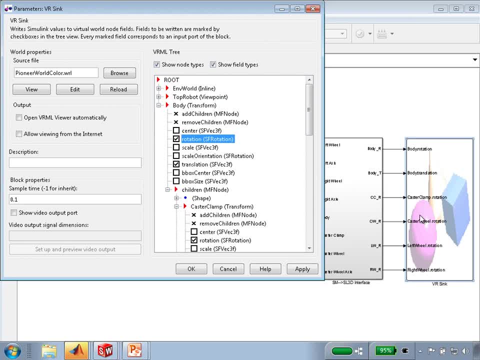 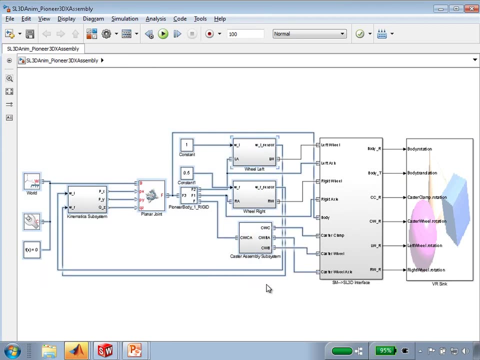 and the translation vector for the body And you have multiple instances of inputs that the VR animation needs here for it to animate the robot. So we have two parts here. We have part one where you have the Simulink SimMechanics model. 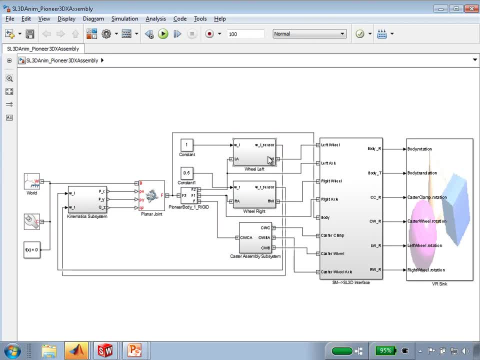 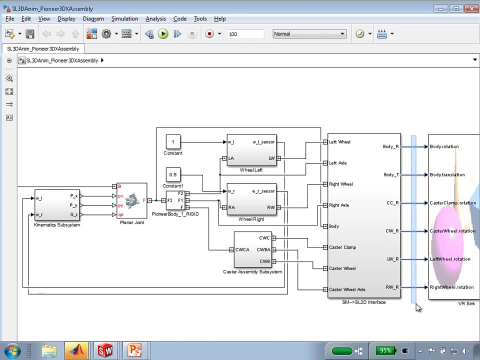 that gives you access to all these coordinate, transforms and geometry here with respect to the robot, And you have part two, which is the VR sync block, which is expecting these parameters. How do we get from part one to part two In order to do this? 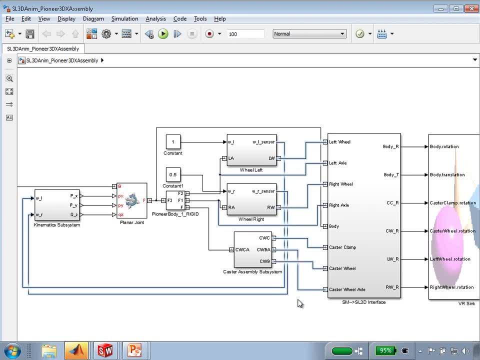 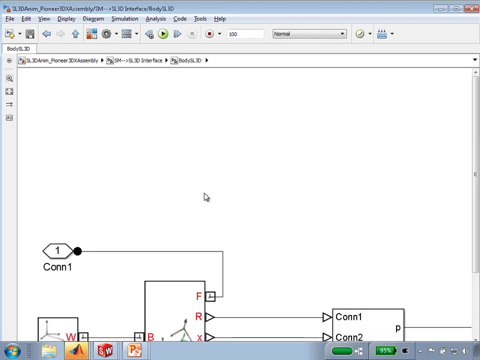 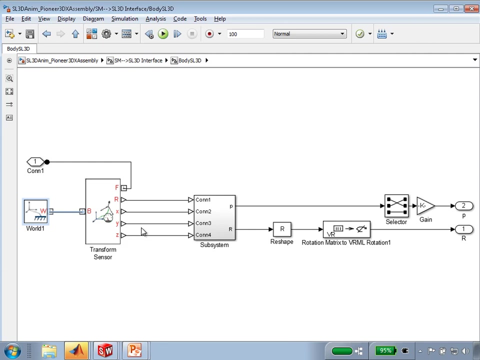 we can use these coordinate transform information and do basic coordinate geometry and transformations to get these information. This is essentially done in the SM-SL3D interface subsystem By use of a block called the transform sensor. Here we measure the coordinate transform with respect to the world frame. 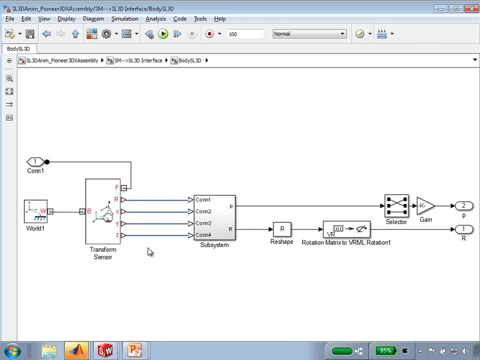 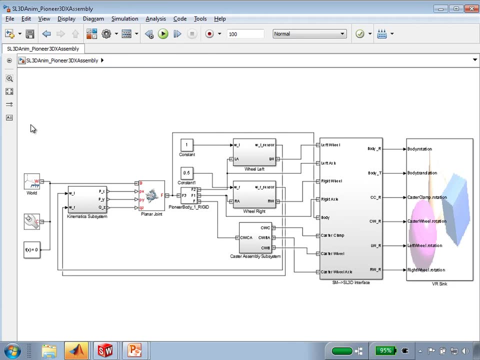 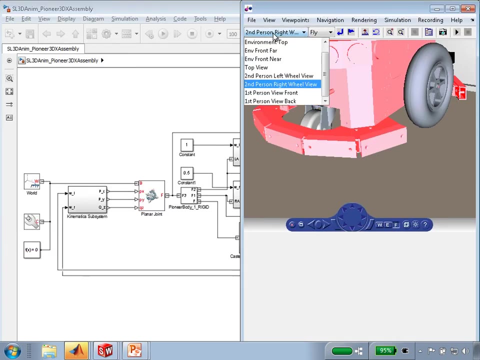 and compute various parameters, like the rotation matrix and the translation vector, and feed it to the VR sync. So let's go ahead and see if we feed this information from the dynamic model to the VR sync. what is the output here? So I'm going to switch to the top view here. 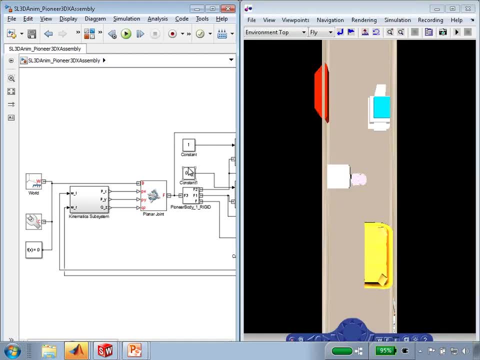 Simulate this model and see what happens. So we see here that the omega L and omega R are 1 and 0.5. so we are expecting the robot to move in some sort of a circular fashion. So we see that the robot actually does that. 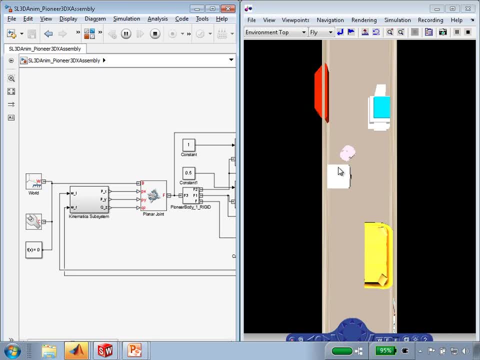 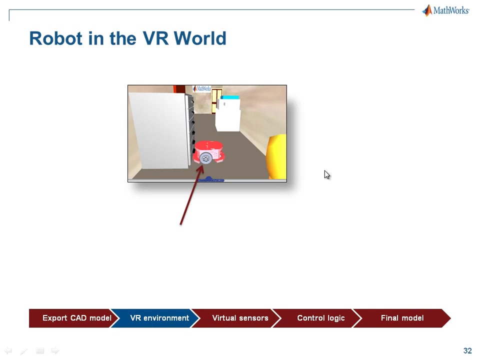 We see that it actually goes through a particular object, but that's fine, because we have not yet implemented our collision avoidance system. This is just to check that the animation works correctly. Let's go back to the presentation to do a small recap. Here is the robot that we got from the export. 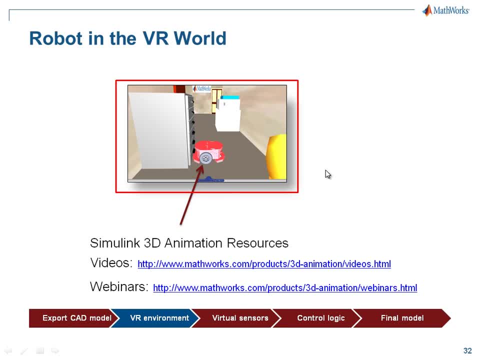 and here is the world here, As I was already saying, we are not going to be focusing on building these worlds in this particular webinar. The MathWorks website already has really good resources for these things. Take a look at the links at these particular resources. 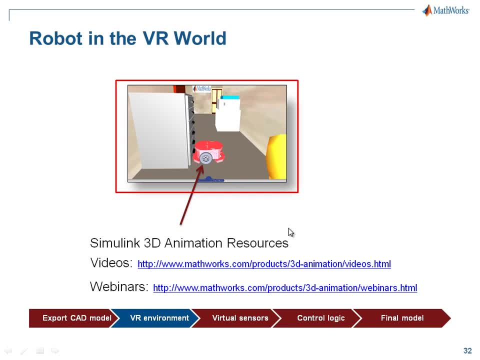 and in order to know more about how you can build custom environments and how you can incorporate the robot model within custom environments. So let's move ahead thinking that we actually have this particular file to work with. Next thing we would like to see is to make the robot move based on our commands. 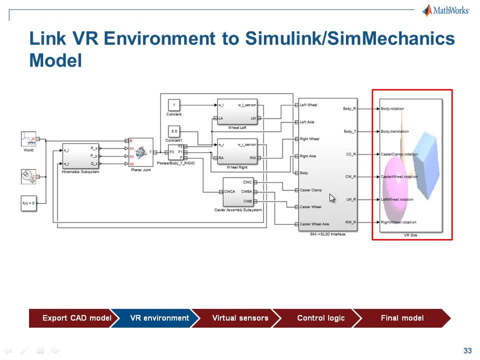 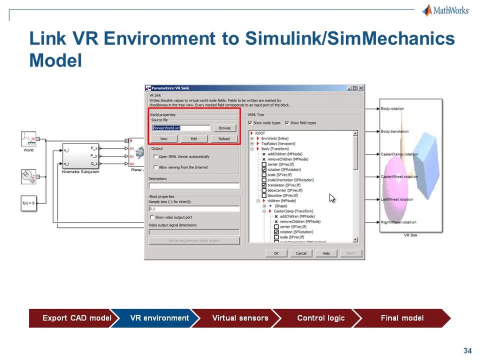 We can link the animation to the Simulink SimMechanics model using the VRSync block. The VRSync block from the Simulink 3D animation library specifies which VRML file to use and since the block itself is in the model, 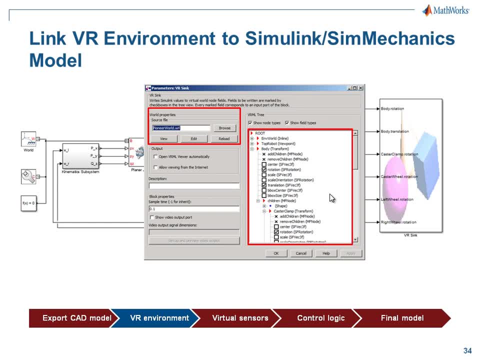 we need to provide it inputs and we choose the inputs in this particular frame. here, In this particular demo, for example, we use the rotation matrix of the body, the translation vector for the body, etc. in order to drive the VRSync block. 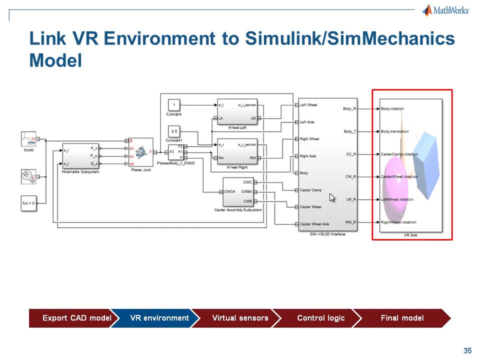 So we have these two parts. The VRSync block waiting for information, like the rotation matrix and translation vector for various bodies. The Simulink, SimMechanics model, which provides us access to various coordinate transforms of the robot. We could simply do certain basic. 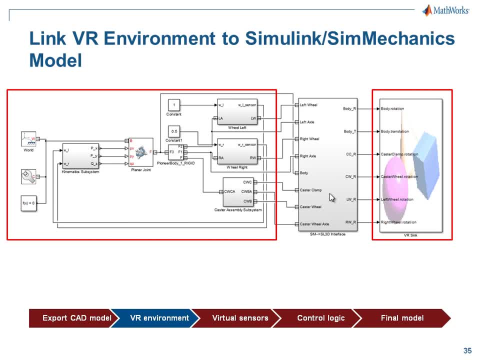 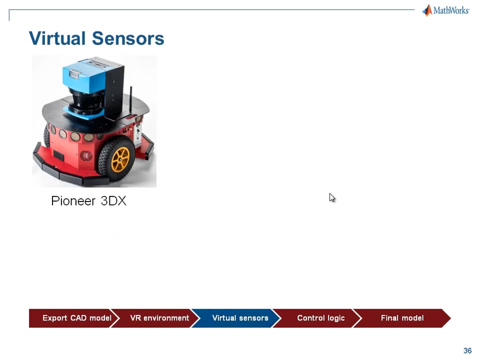 coordinate geometry and transformations to get from one point to another. The transform sensors in the SimMechanics library can be used to do this. So inside the SMSL3D interface subsystem we implement this. So once we have this animation interface ready, 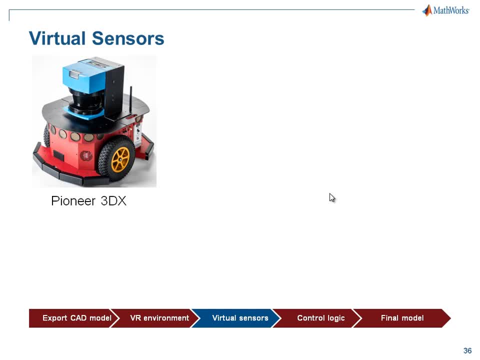 let's talk about sensors In the real world. we have actual sensors to work with Actual physical sensors, We have a physical signal based on some stimuli. So in the image we actually see the Pioneer 3DX robot from Adapt Mobile Robots. 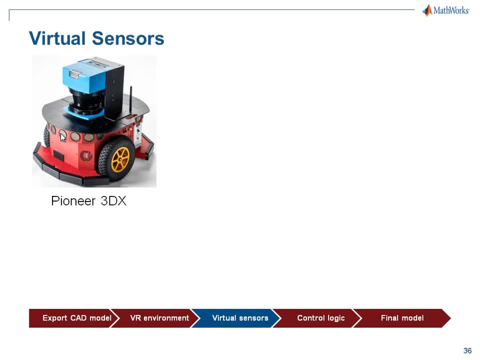 This is a very robust and versatile robot which is popular in the academic research platform. This particular robot has sonar sensors in the front and the back. It also has front and rear bumpers. This particular robot also has a lead arm mounted on top of it. 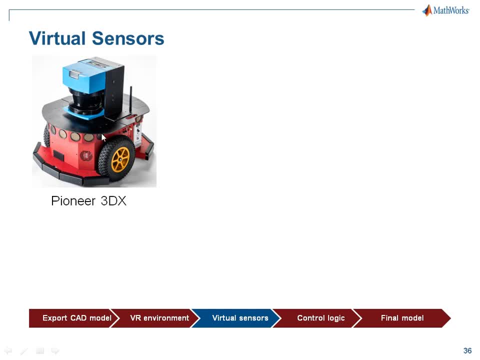 For our collision avoidance demo. we are going to just use the front eight sonar sensors. However, you could use this particular approach to model and implement different sensors for a more complex algorithm, But the fact is, in simulation we need to model them in some way as virtual sensors. 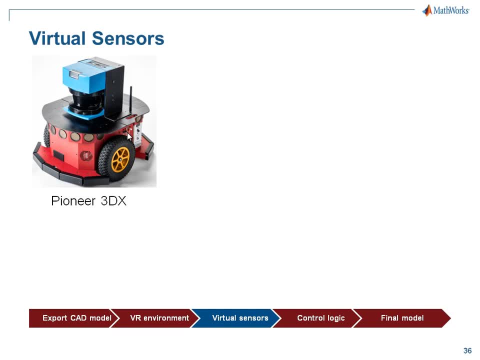 so that our control logic can react to it. in simulation, Here is how our sonar sensors are arranged from the top view, And if these are the sensors, this is where they are actually located in the real robot Now, at any given time. 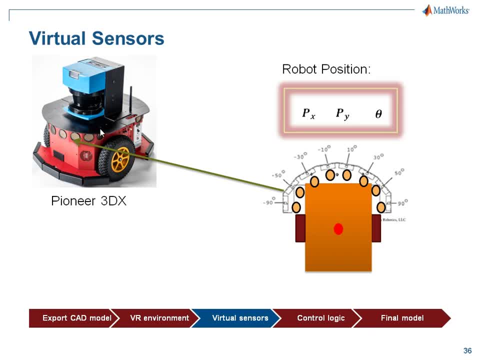 we know the position of the robot given by Px, Py and Theta. Based on these values, we can determine the position of each of these sensors with respect to the world. So as the robot moves in the world, we can also get the x and y position. 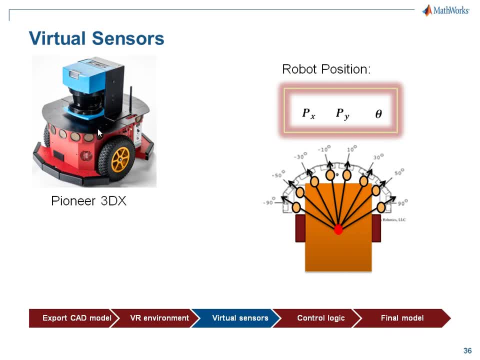 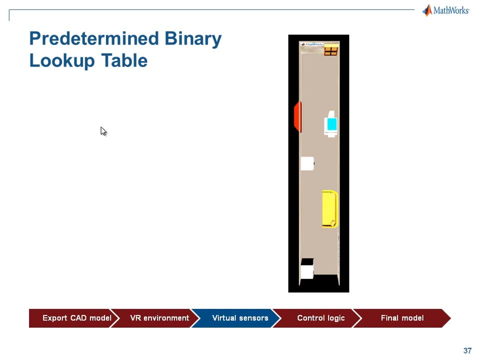 of each of these sensors in terms of the absolute world coordinates, etc. So if we have this custom virtual environment in this example, it is a binary lookup table that we can develop. wherever there are objects, you have a one, and wherever there are no objects, you have a zero. 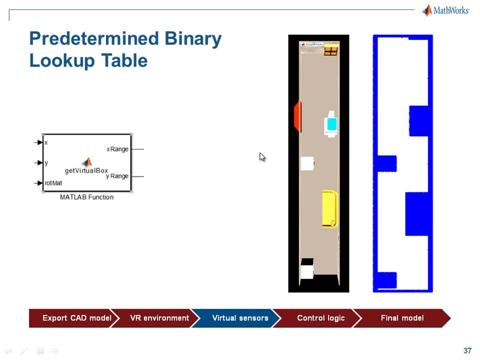 We have already established that, given the position of the robot, we can get the sensor position Using this sensor position and this world map that we already know. we can get a simple obstacle distance from a given sensor by looking up the distance with respect to the table here. 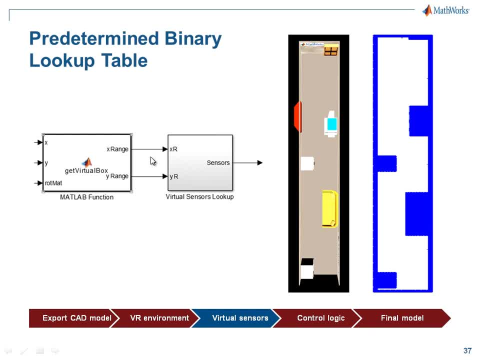 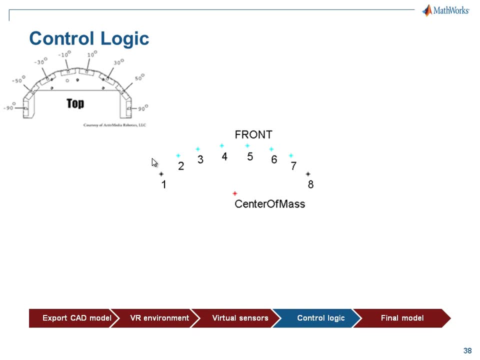 So we get the sonar value for a given sensor, given the position of the robot. Once we have the sonar values, we need to see how we can do control logic. for this We can do a basic MATLAB plot like this to understand how the virtual sensors are arranged: 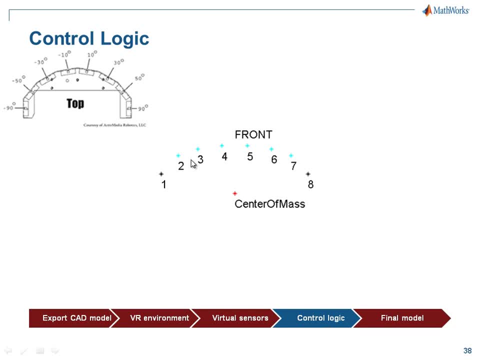 For the collision avoidance algorithm. like I said, we are going to use only the front eight sensors. When sensor one detects an object, we are going to perform a turn right wide operation. We are going to couple the sensors two and three and if either of these two sensors detect something, 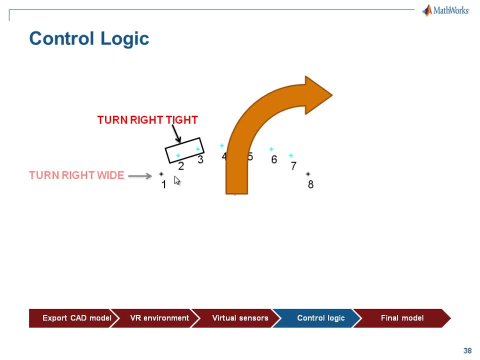 we are going to do right, but this time in a tighter radius than before. Similarly, we combine sensors four and five to be the front sensors. If either of these front sensors detect an object, we are going to rotate in place and based on the magnitude of these two sensor values, 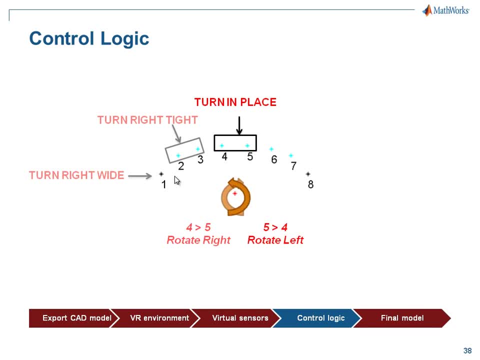 we decide whether to rotate left or right. We can follow this symmetry and do a turn left- tight operation and turn left- wide operation. for the rest of the sensors, It is important to note that in this approach we deal with the first object we detect. 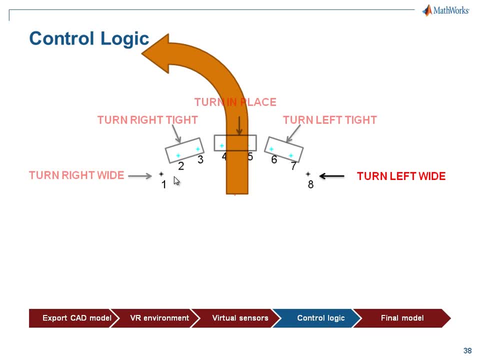 and take necessary action In case two objects are detected at the same time by two sensors. we give preference to take corrective action for the front sensor and then move outward as preference decreases. This is because the corrective action for the front sensors is the most aggressive. 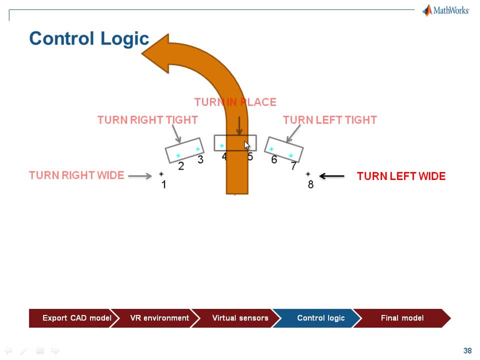 and performing that will definitely avoid objects detected by other sensors as well. Here we can also imagine that the robot is going to be doing one of these operations at any given point of time. We can also think of them as states, so the robot could be living in one of these states. 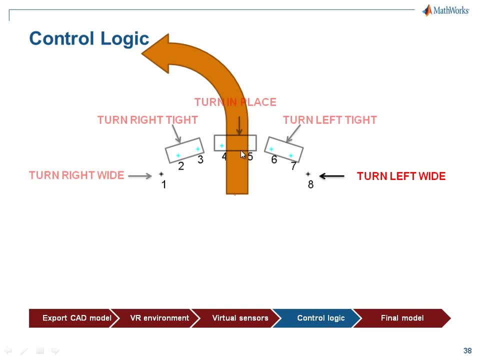 at any given point of time. With this information about the sensors and the control logic, let's take a look at how these were modeled in our Simulink SimMechanics model. I'm going to go back to MATLAB and pull up the model where this was implemented. 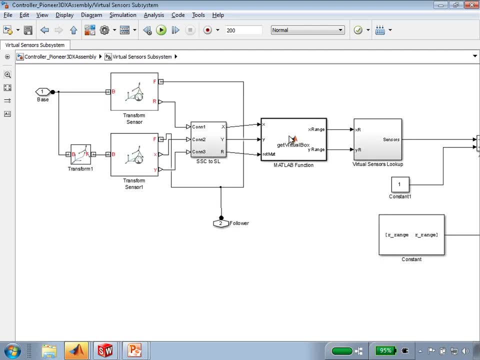 So let's take a look at the virtual sensors first. So, given the x, y and the theta information from the robot, you can get the x and y position of every sensor, And we use a MATLAB function in order to get that information. 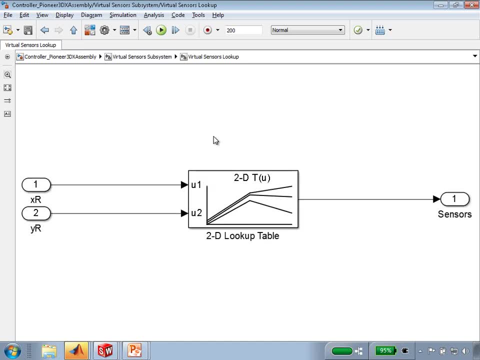 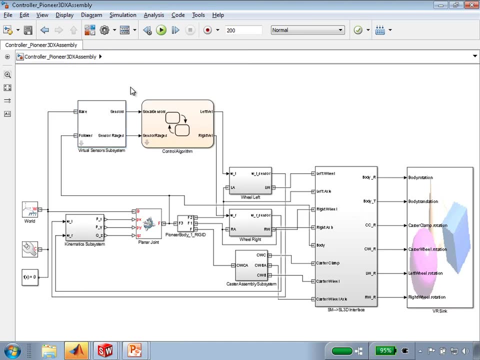 Once we do that, we can do a simple lookup table to get the sensor values. Once we get the sensor values, the next thing we need to work on is the control logic. State flow was chosen to implement the supervisory logic. We could have very well written. 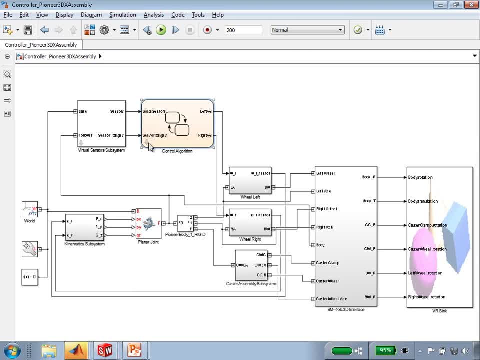 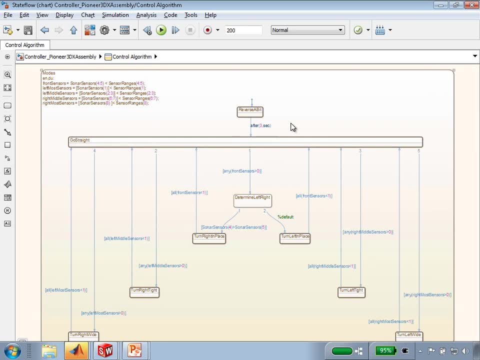 if-else and switch-case MATLAB code to achieve this, We use state flow because it's a high-level graphical language which makes it easier to understand than low-level code using if-else conditions As an example. in this model, the modes of the robot are modeled. 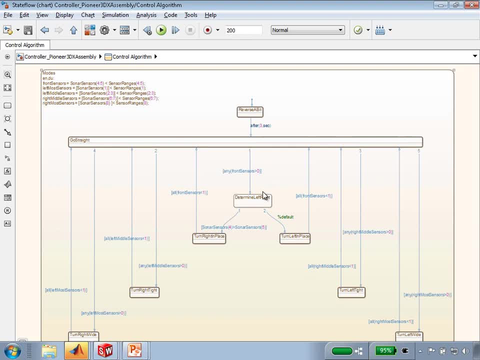 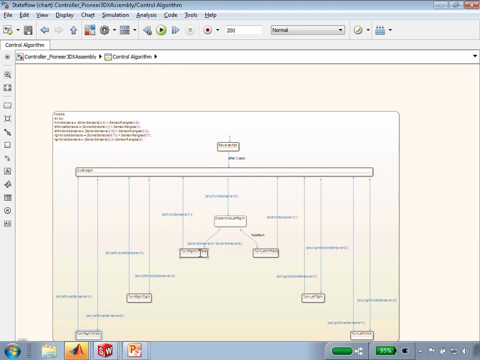 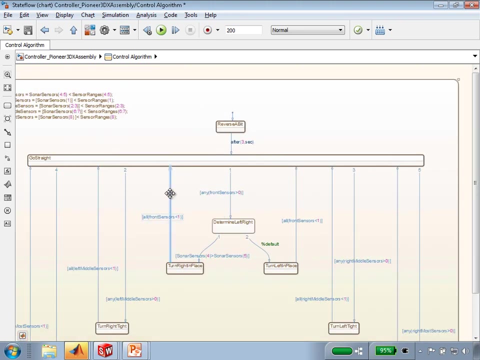 using rectangles called states. For example, here is a state where the robot is going to turn right-wide and here is a state where the robot is going to turn right-in-place. Apart from this, we also have these arrows which point to transitions. 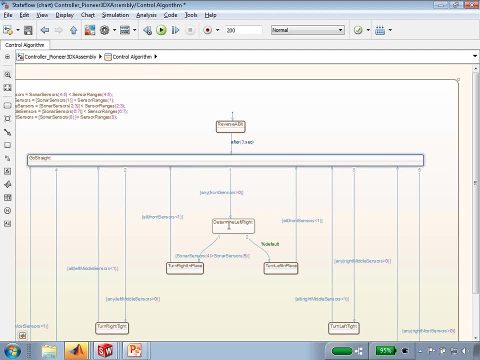 These arrows determine when you move from one state to the other. For example, this transition says move from go straight to determine left-right when any of the front sensors are detected. This would have been harder to understand using if-else and switch-case conditions. 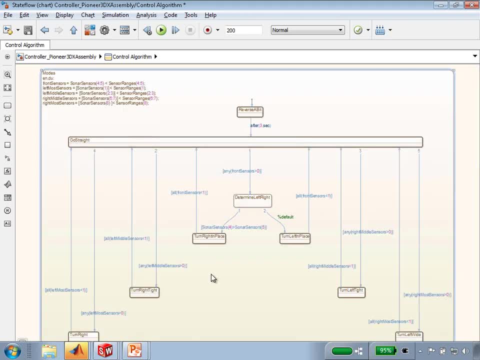 Apart from this, state flow also has a built-in debugger and animation that can help you debug logic. I will show this to you a little later, when I actually demo this model to you. If you are new to state flow, I would encourage you to take a look at. 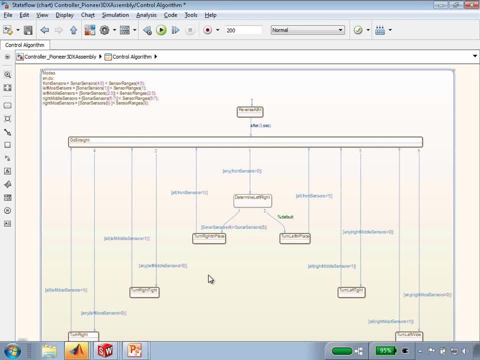 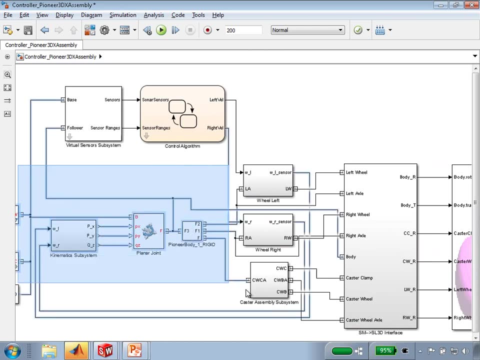 the getting started with state flow webinar in the state flow product page. Now, after all this, our final model looks like this: You have this part, which is the part one of the webinar series, which is the Simulink SimMechanics model. 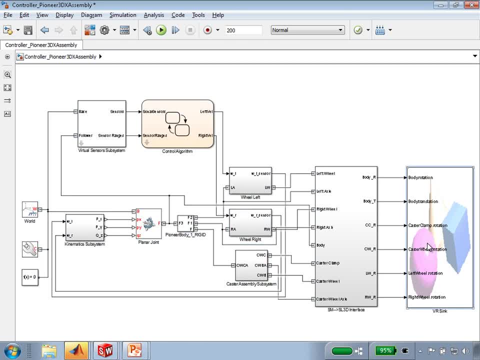 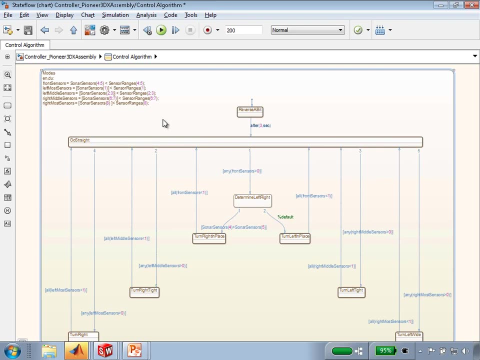 You have the VRSync block which provides the animation information. You have the interface here which links the Simulink SimMechanics model to the Simulink 3D animation. You have the virtual sensor subsystem here and you also have the state flow control logic here. 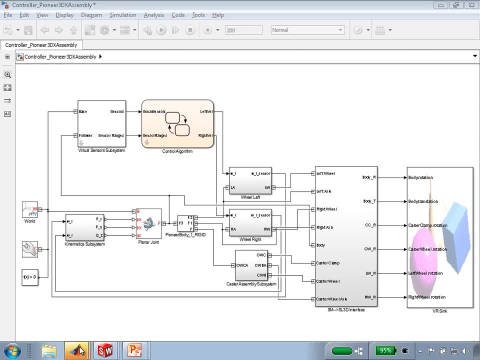 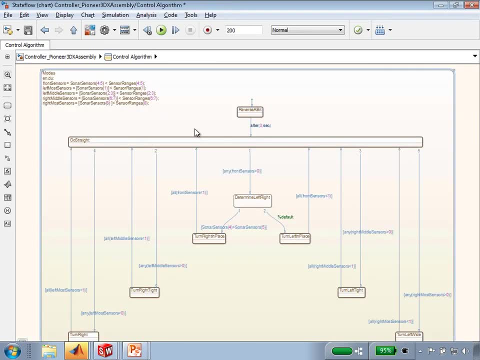 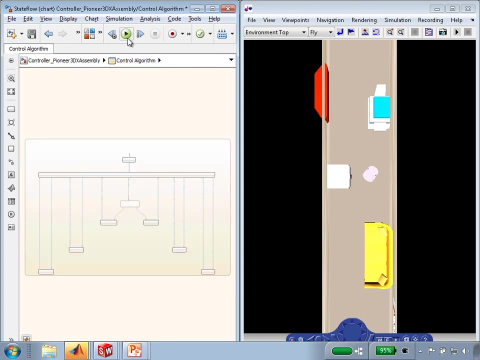 Let's see, when we simulate this model, what happens. So let me pull up the animation window here on this side and let me also have the state flow on this side and let's see what the robot does under different conditions. So let's hit play and see what the robot does. 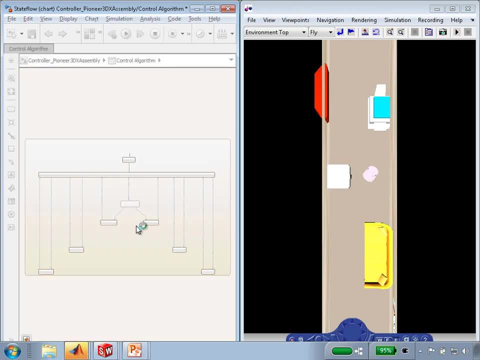 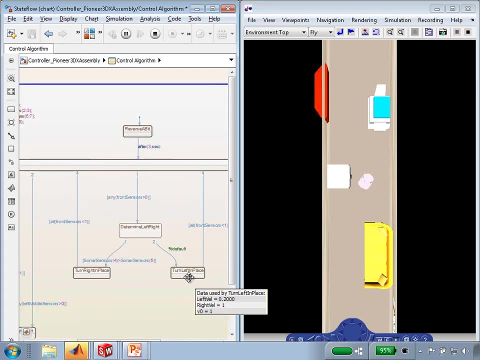 under the various simulation conditions. So you can see that the robot is in the reverse a bit state. Now it has moved to the turn left in place and you can actually see that the robot is moving under different states based on what it wants to do. 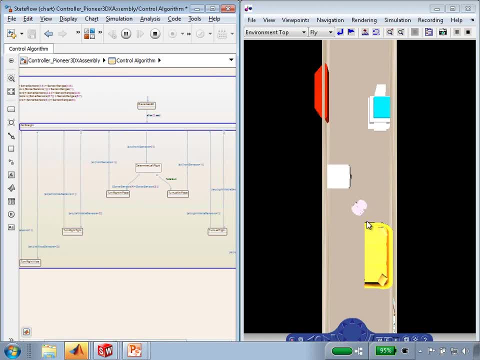 based on whether it's moving, looking at an obstacle, or whether it's moving straight, etc. And with respect to Simulink 3D animation, you can actually change these viewpoints. So, for example, right now I can sit on top of the robot and see what the robot does. 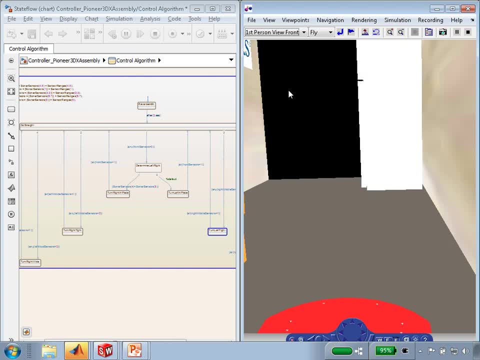 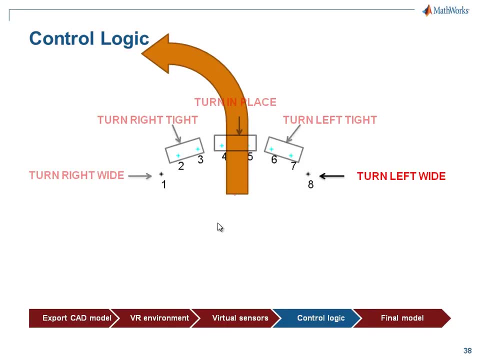 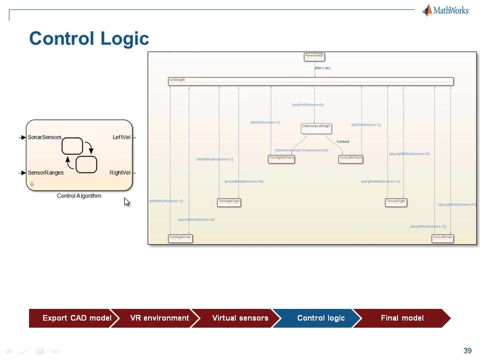 and visualize the dynamic system and debug my control logic as well at the same time. Let's go back to the presentation to do a recap. We model the control logic instead of the state flow, as its graphical representation, with state machines and flow charts, is easier to develop and understand. 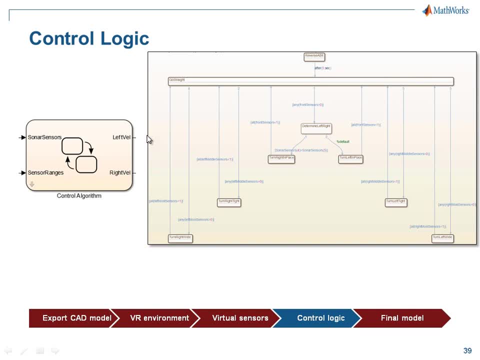 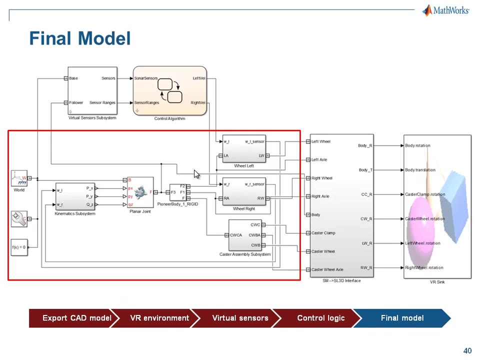 The control logic takes sensor values and ranges as inputs and sets the wheel angular velocities as outputs. You can find resources to various videos and webinars, specifically with respect to state flow, at these links. Our final model looks something like this: The Simulink SimMechanics model from the CAD import. 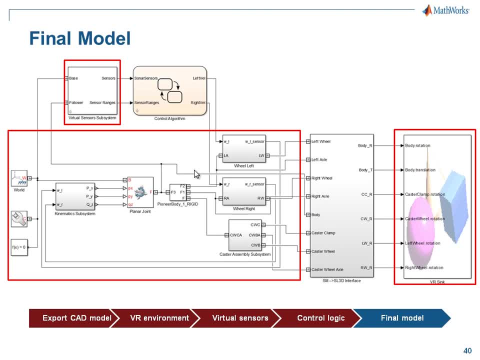 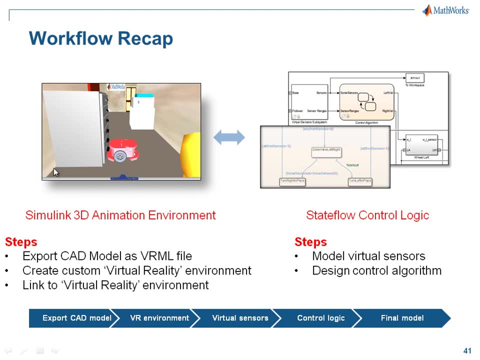 the VR environment, the virtual sensors and the control logic. here To recap the workflow: we started with the CAD model and exported it to a VRML file, Then we created a custom virtual reality environment for the robot to live in And finally, we saw how we can use the VR sync block. 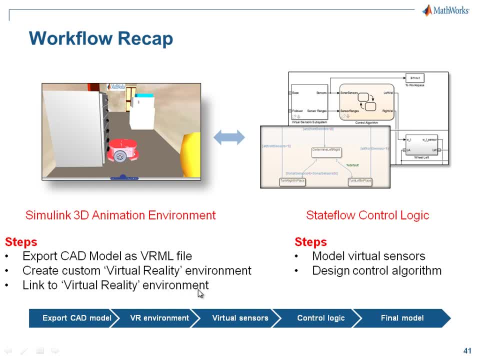 to link the virtual reality environment to the dynamic model. Then we went to the control logic part, where we model virtual sensors using lookup tables and then designed the control logic using state flow. So now we have a controller which works well in the simulation environment. 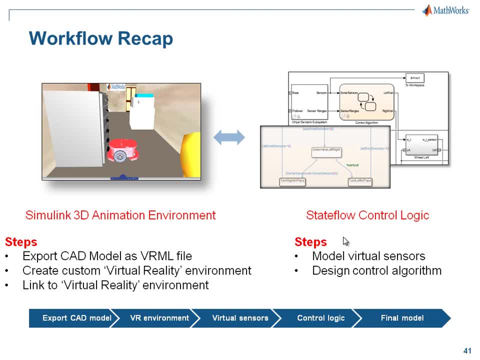 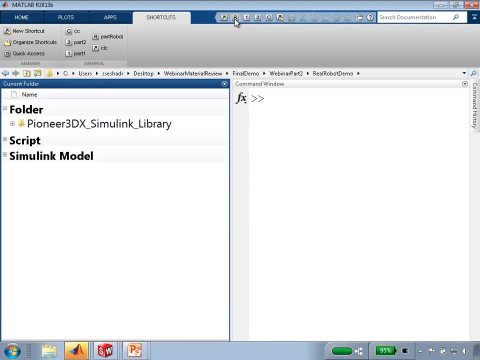 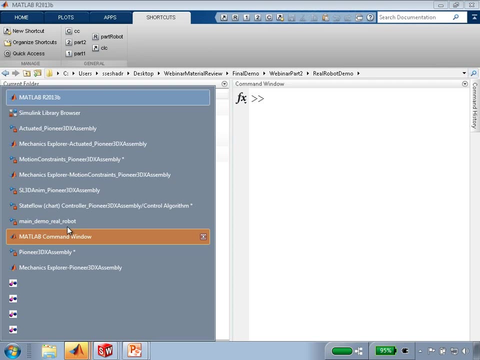 Where do we go from here? How does this translate to a real robot? Let's get back to MATLAB For Simulink. to communicate with a robot, we need some sort of a model to talk to the robot. Here is a model which can talk to the robot. 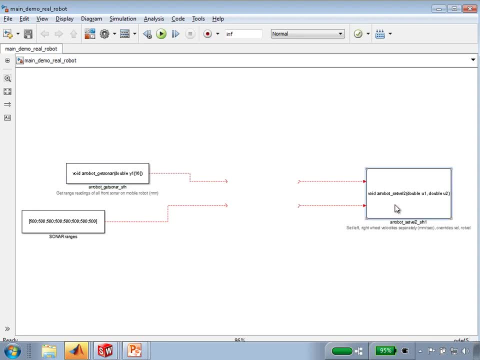 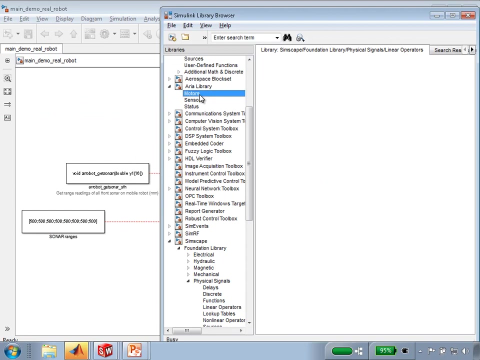 Here we are using these blocks that were actually developed by ADAPT and made available for use within Simulink, to talk to the Pioneer 3DX model. These blocks come from this library here and you can see that the library has several blocks which are called as motors, sensors and status.